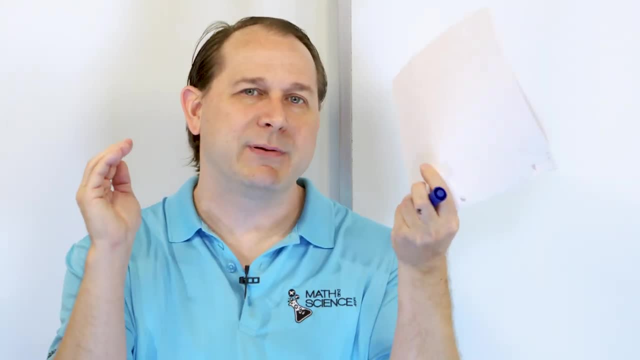 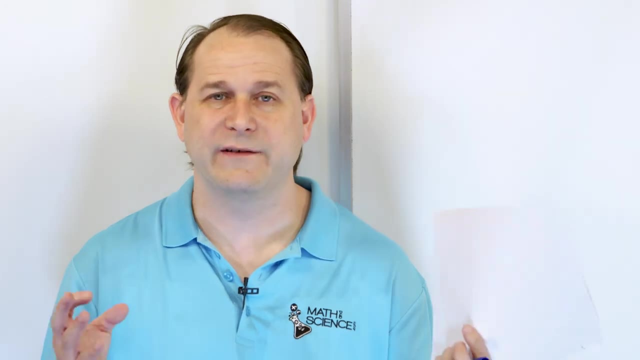 multiply it out by hand, but it's a giant pain. What if you have A plus B raised to the 17th power? Tons of multiplication you'll have to do by hand. It'll take pages of work to get the answer. This lesson is going to show you how to get those answers really really, really fast. 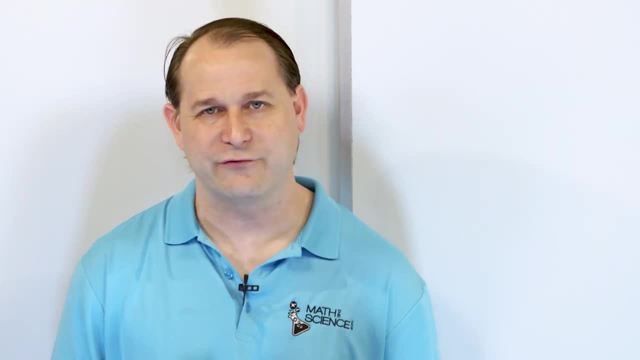 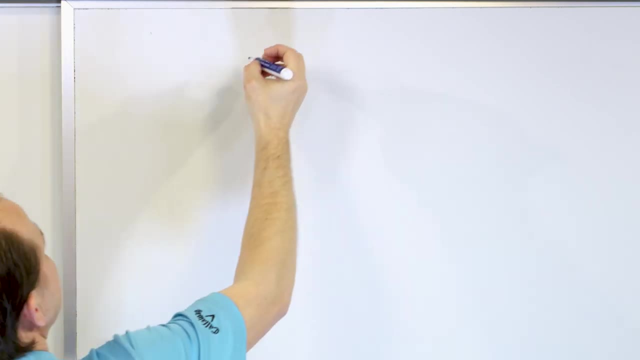 And in order to do that, we need to understand something first called Pascal's Triangle. So let me introduce that first, and then I'll connect the dots and show you how we're going to ultimately use it. Here we have Pascal's Triangle. Obviously, the triangle means 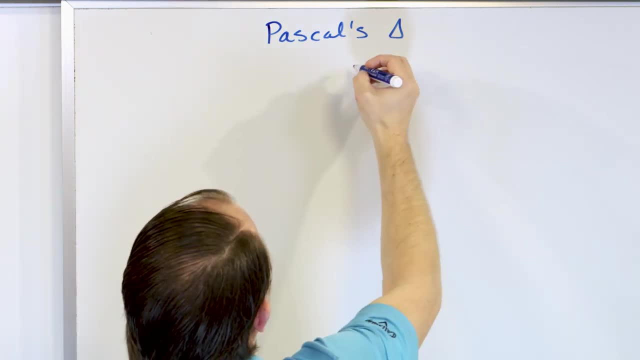 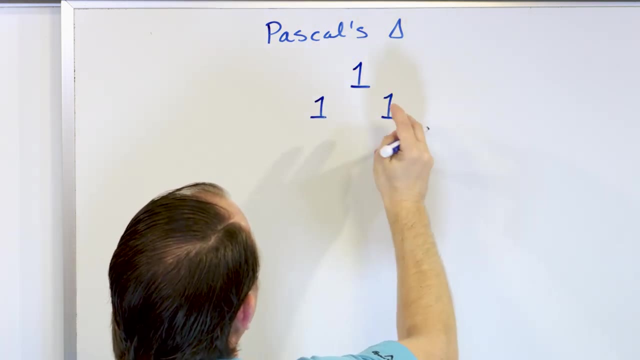 triangle. All right, here's what you do. First, to start the triangle off, you put a number one right here, okay. And then to the left and to the right of that one, you put another number one and another number one, So you kind of make a little triangle of ones. This is how it begins, It always. 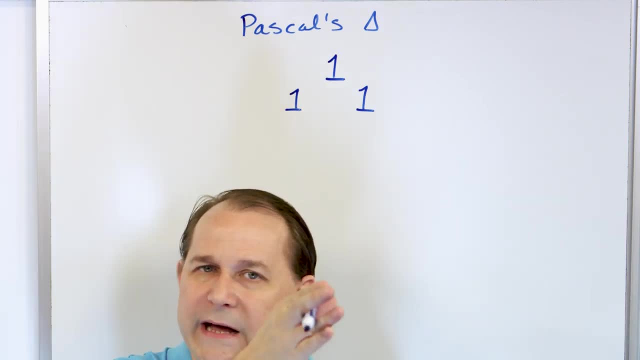 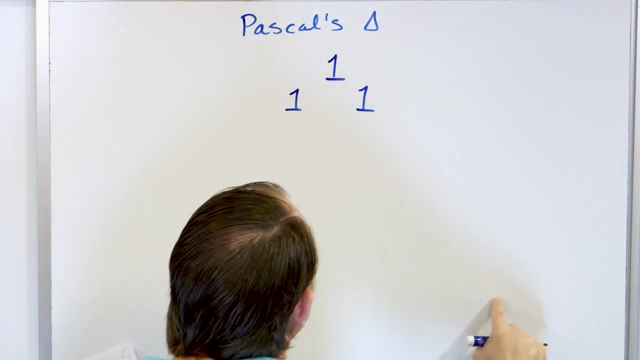 begins the same way: One on the top, flanked right underneath by another one, and another one. okay, Next, in the next row, you go down to the left. See, all the diagonals here of this triangle are all going to be a one. You'll see why. 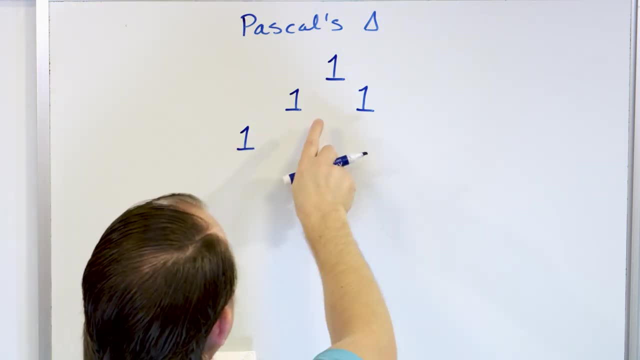 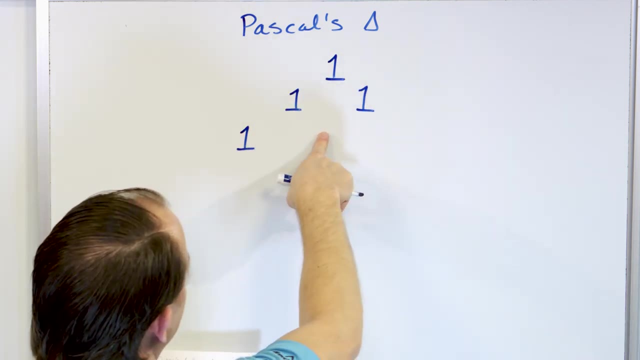 in a second, but put a one right here Now to get the number that goes over here, because this is one line, one element, two elements. See, this is going to be three elements. To get the one in the middle here, what you do is you look at what's above it and you add them up, So one plus one. 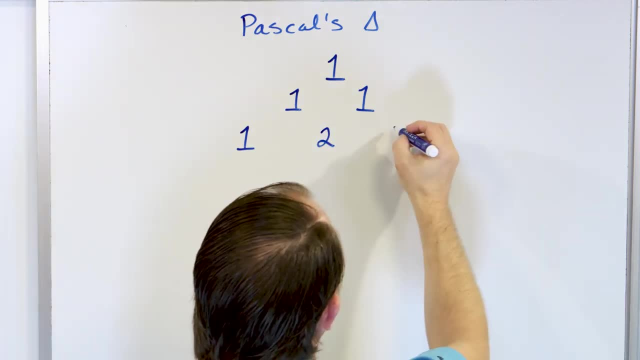 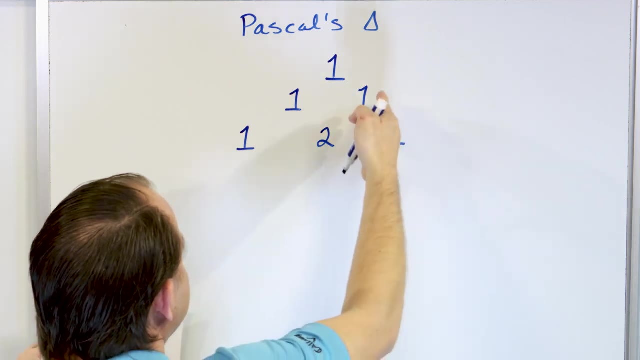 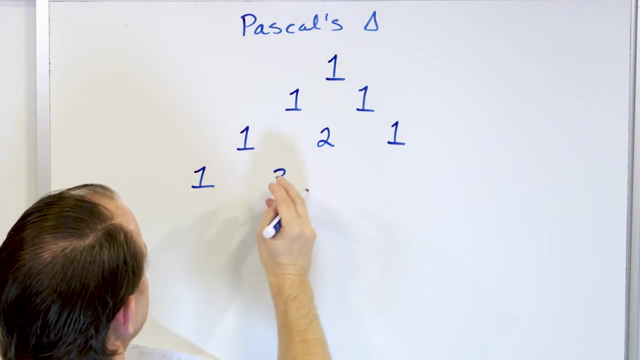 is two. So we put a two right here And then off to the end. the edges of the triangle always has elements To go to the next line of the triangle. we always start it with the number one And then to get what goes between these guys, we add them up. One plus two is three And then we skip over. 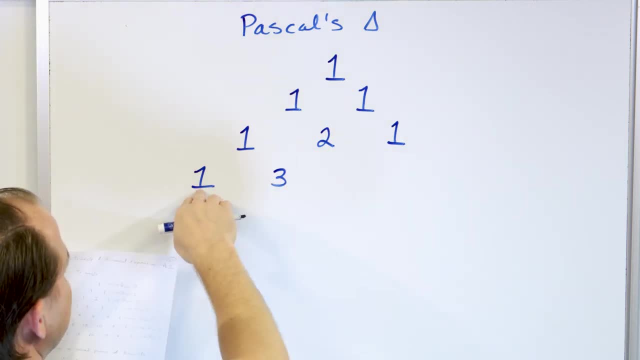 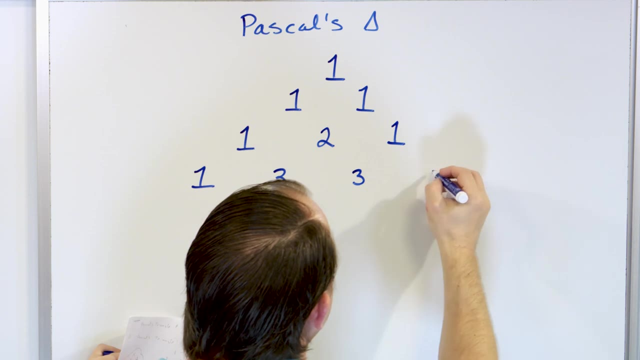 this to this spot here, because we're only really putting numbers in the kind of in the spaces between the numbers above. So we skip over here. One plus two again is three, And then on the edge of the triangle we always put a one. So you see, to formulate a Pascal's triangle, all you're doing. 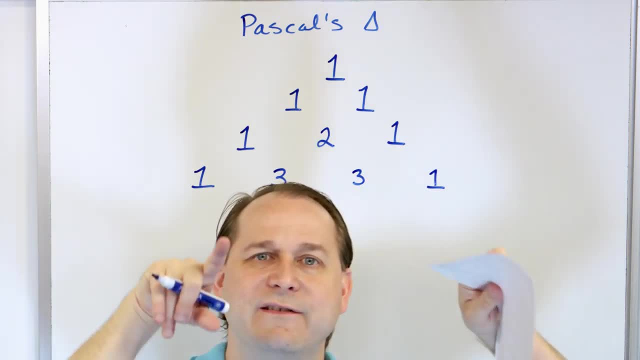 to write the elements of the next line is you're just adding up the two numbers that are directly kind of above it into the left and to the right. So to go to the next line again, you always start it with a one. So put a one there And then to plug a spot into this location, it's. 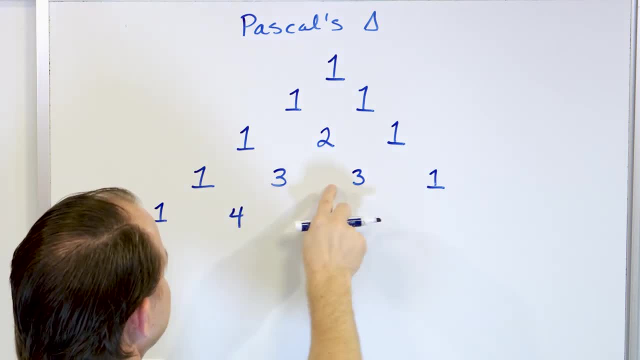 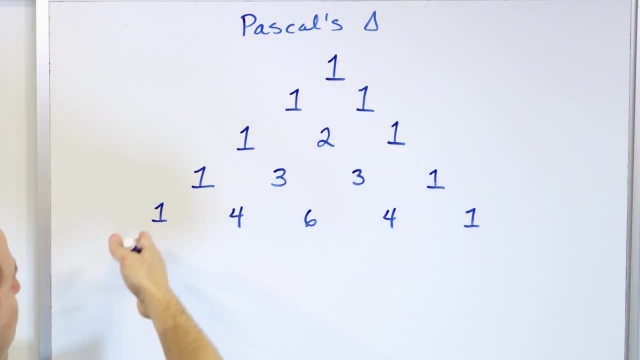 one plus three, which is four. To put a spot here, it's three plus three, which is six. To put a number here, it's three plus one, which is four, And then on the end you always have ones, always. 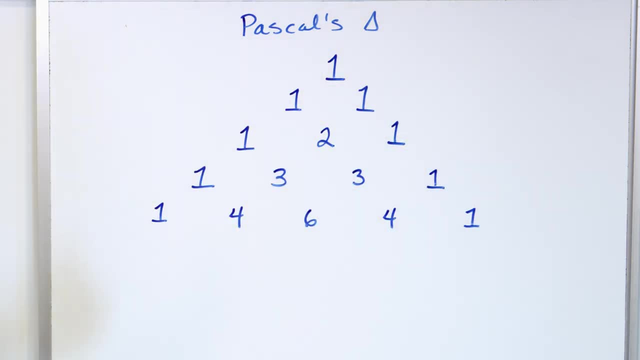 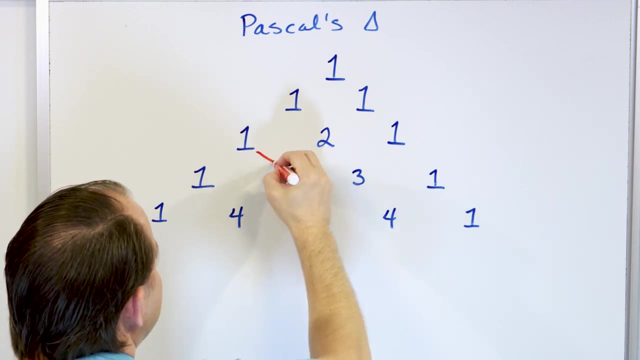 on the edge of the triangle. Okay, we'll do two more lines just to show you how it works. But before we get too much farther, I'm going to draw a little, a little line here and then I'm going to start showing that to get the number three here, what you're doing is you're adding a one. 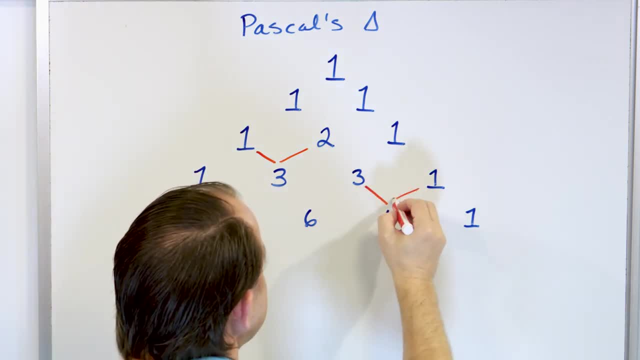 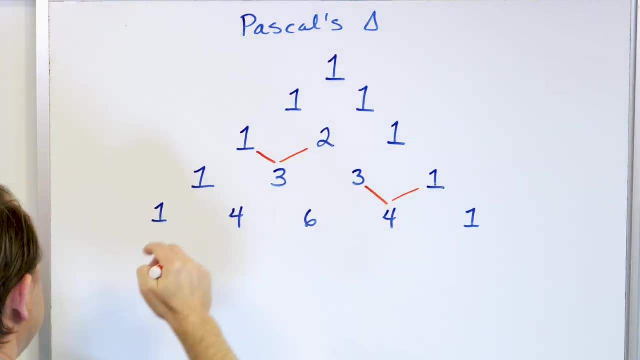 plus two To get the number four. here what you're doing is you're adding the three plus one. So I'm not going to draw these little things everywhere, but these are how you're getting the numbers. This would form a little little triangle like this and so on, showing you how the addition 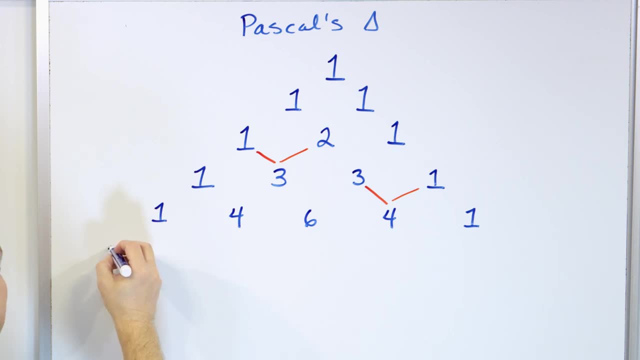 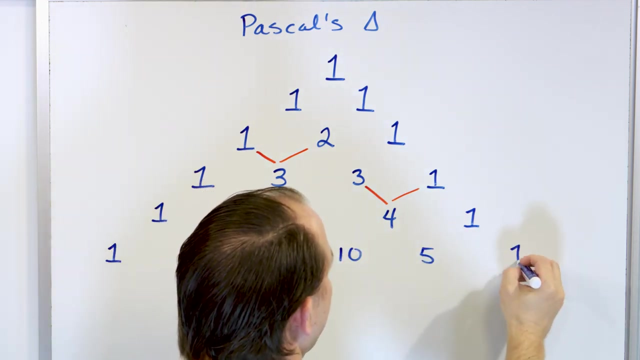 happens. We'll do two more lines and then we'll kind of talk about how this is useful for doing algebra here. So in the next spot it's one plus four is five. In the next spot, four plus six is here, four plus one is five. and then here we have a one, always on the edge, the last line that we 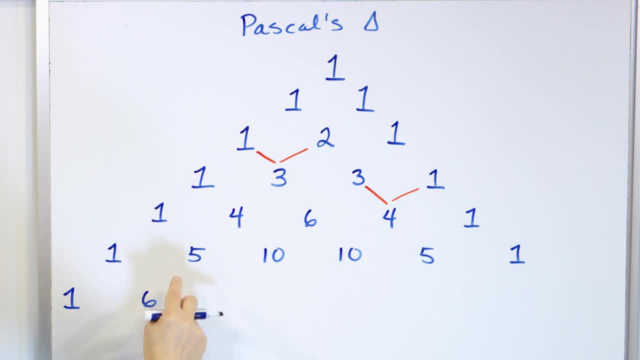 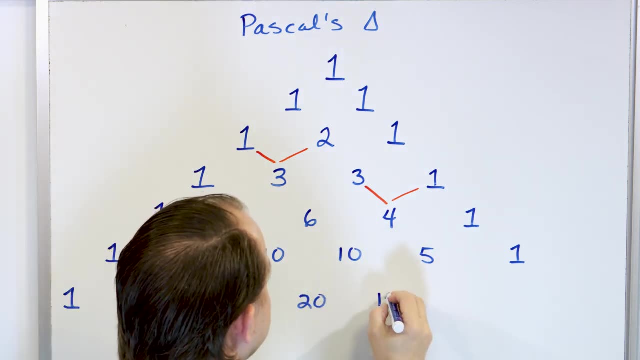 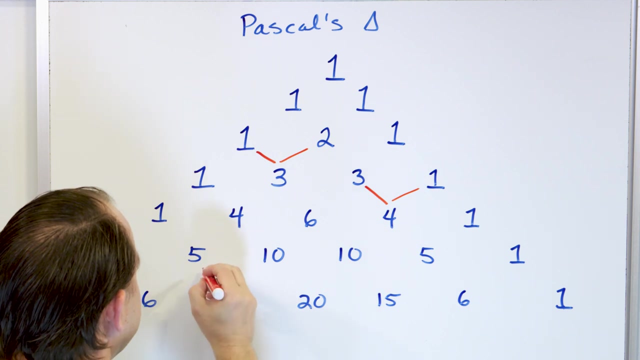 will do. we always have a one in the diagonal. one plus five is six. five plus ten is fifteen. ten plus ten is twenty. ten plus five. fifteen, five plus one, six, and then always a one out here and again just to drive it home. to get, for instance, this one, you're adding those two. 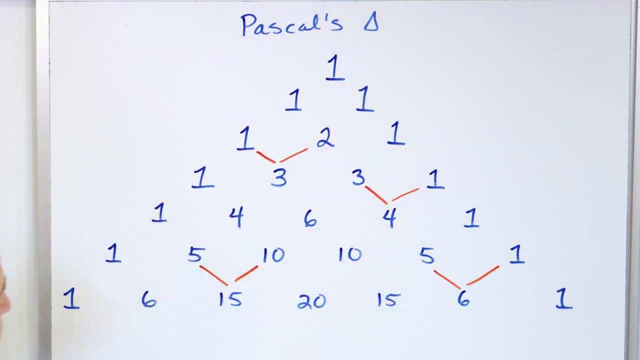 numbers together, for instance, to get something like this: you're adding these two numbers together. that's how you get. so let me spend just a second double checking my triangle: one one one, one, two. one one three. three, one one four, six, four, one one, five, ten, ten five one one, six, fifteen twenty. 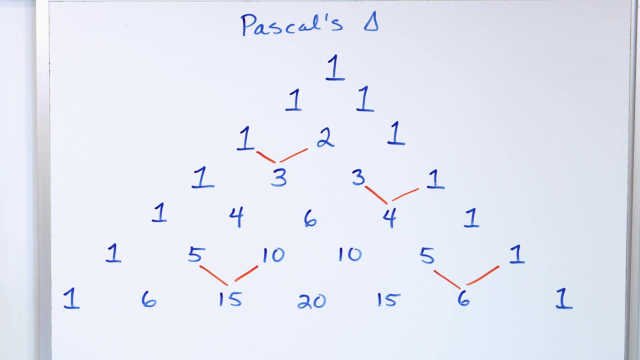 fifteen, six and one, that's correct. so a couple things i want to point out before we go any farther. first of all, notice that you can generate any number of rows of this triangle that you want to. right now we stopped right here, but if i need you to go one more level deeper, you could easily. 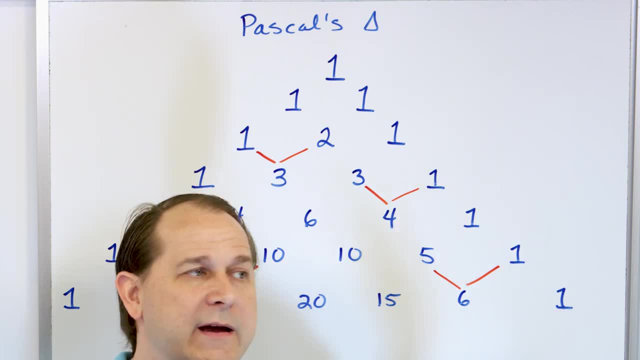 do it by just adding the appropriate spots in the triangle, uh, to the triangle, and then you can just add the appropriate spots in the triangle to get the next line and then the line after that. we would just add the numbers right above it, and so on. 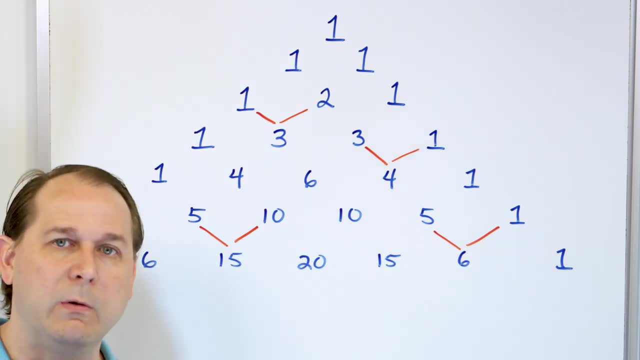 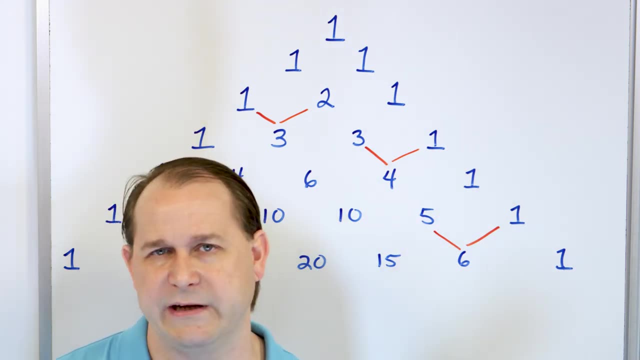 So if I wanted to get the 100th row of this table, I would have to generate all the rows in between, but eventually I could get down to row number 100 just by addition. A computer could do that pretty easily, right. 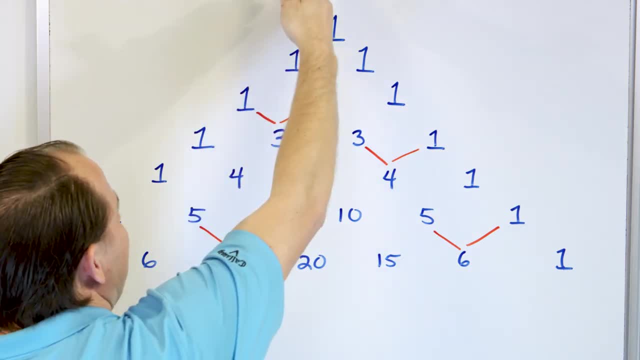 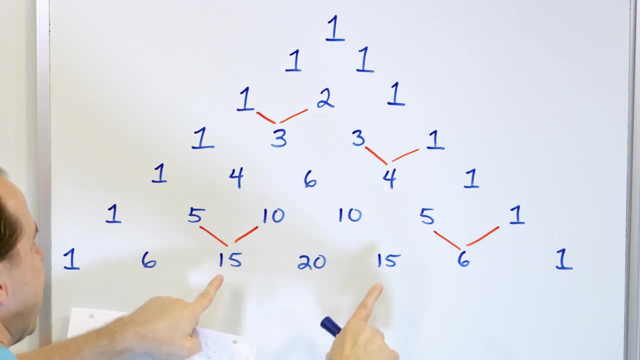 More importantly than that is notice that this thing has symmetry. If you cut a line right here in the middle, then the numbers to the left and the numbers to the right are mirror images. Here you have 15, six, one for that row. 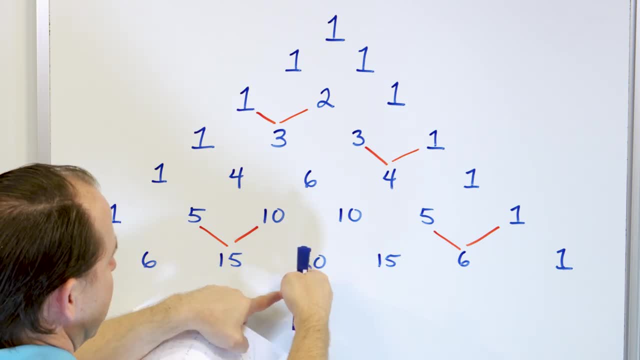 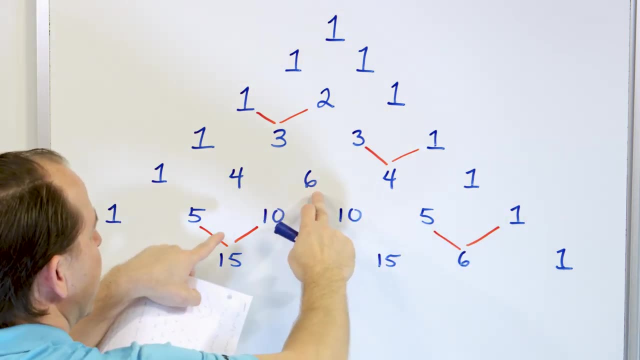 Here you have, and the 20 was in the middle, so it doesn't really have a mirror image. but here there is no middle number. So 10 is a mirror, five is a mirror, one is a mirror Again, six is in the middle, so it's not a mirror. 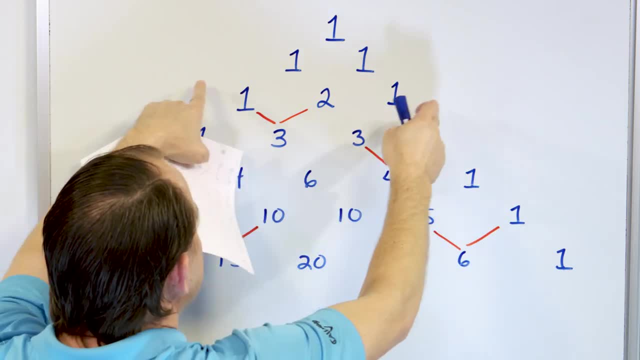 but on the other side of that four and one, you can see the three, the two and the one and so on. So everything's a mirror image and that's always gonna be the case. The right side of the triangle should be exactly the same numbers. 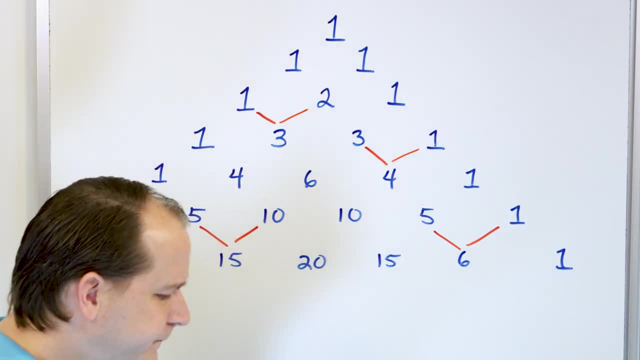 as the left side of the triangle split right down the middle. all right, Now the last thing I wanna do is I want to label the rows of this thing Now. I know you won't quite understand why just yet, but I promise you in a minute. 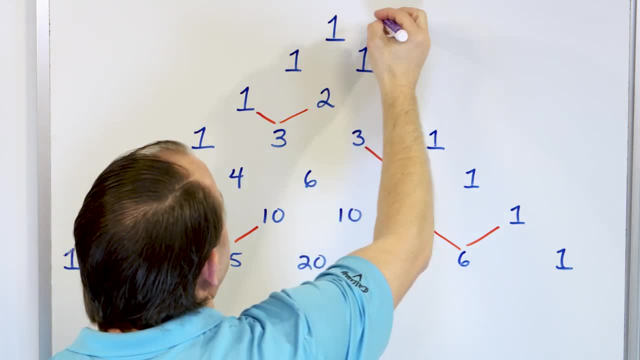 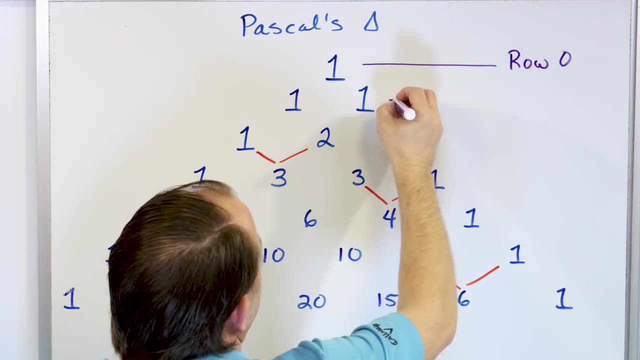 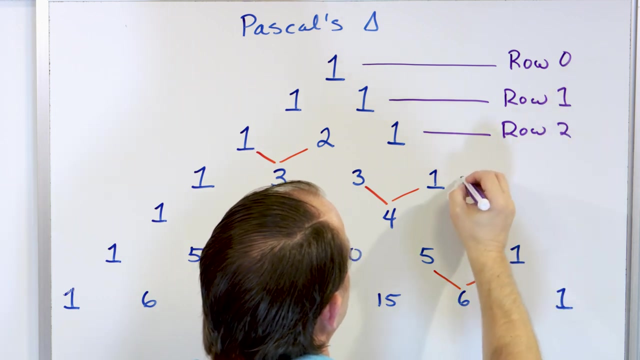 there'll be a really good reason that we're doing this This first row here. even though most people would call it row number one, we're actually gonna call it row zero. okay, We're gonna call this one row one. We're gonna call this one row two. 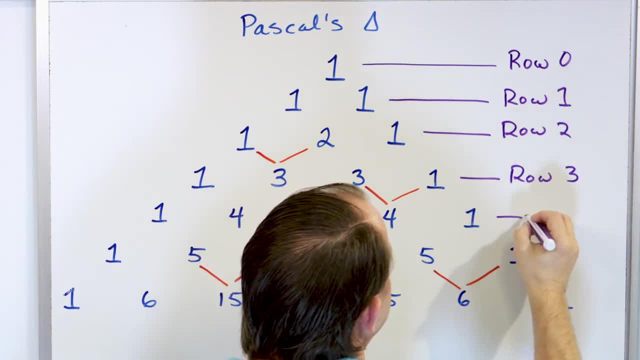 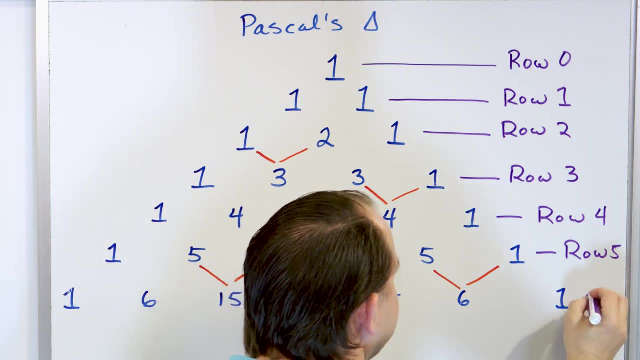 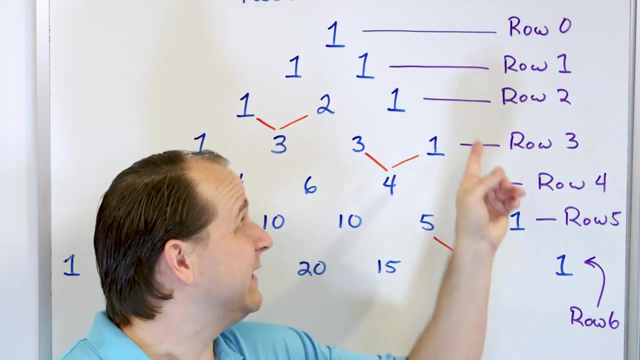 We'll call this one row three. We'll call this one row four. We'll call this one row five, And then this one right here. we'll call it row six. Now again, I'm gonna show you and tell you exactly why we're labeling. 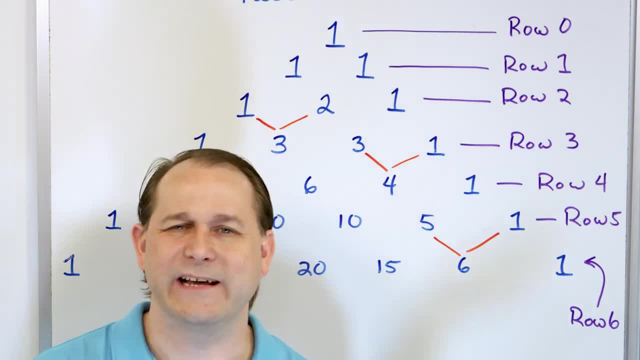 the first row zero instead of one. but it's just gonna get confusing. Just let me get into the meat of it a little bit more and you'll instantly understand why we call that row zero. Now this is a neat little game, mathematical game. 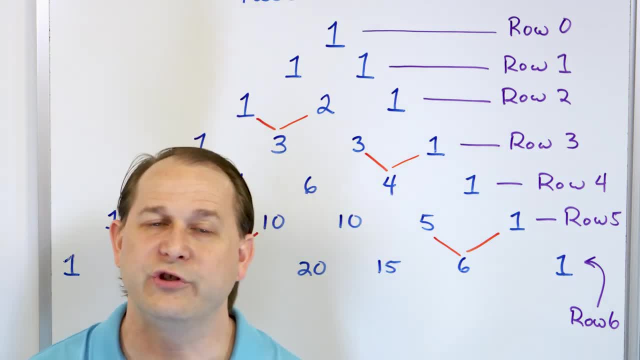 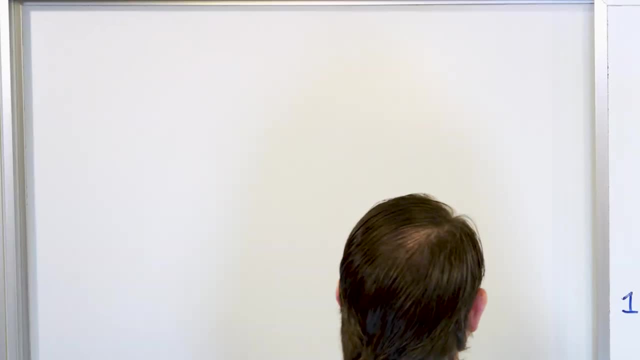 You can construct this triangle. Pascal's triangle has a lot of uses. The use that we are gonna use it for we are gonna use it for is to help us expand binomials. So what I want to do is go down memory lane with you. 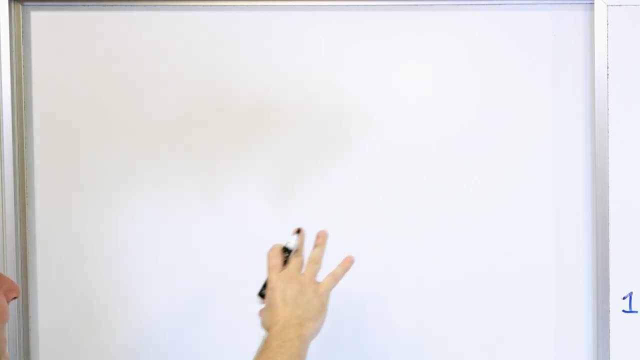 and expand a few simple binomials And we're going to use that to generate a general way to expand any binomial with any power using Pascal's triangle. So, for instance, if we want to expand a plus b to the power of zero, what's the answer? 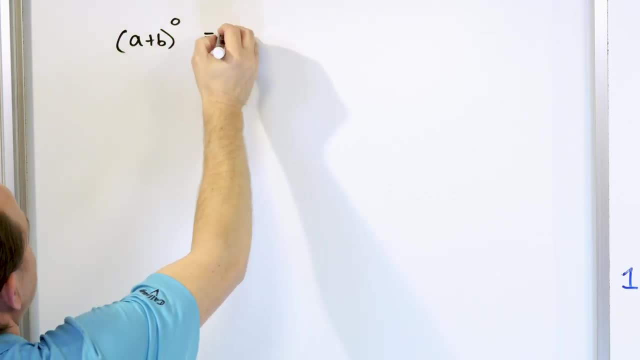 Well, no matter what a and b are, it's raised to the zero power, so it's equal to one. okay, What about a plus b, raised to the first power? Well, if it were squared, it would be multiplied by itself again, but it's just the first power. 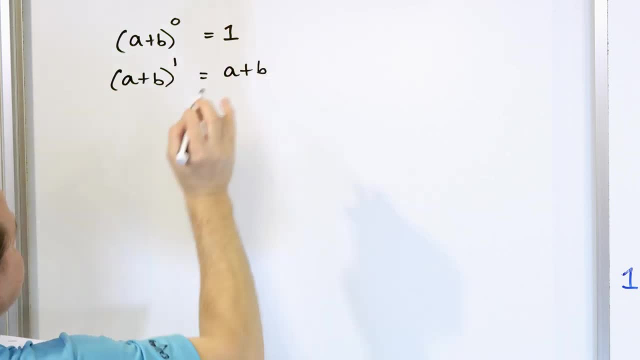 so really, what you get here is just a plus b. okay, So far this stuff is really easy. You're saying, why is he going through this? Well, let's continue on down through here. What if you do a plus b, quantity squared? 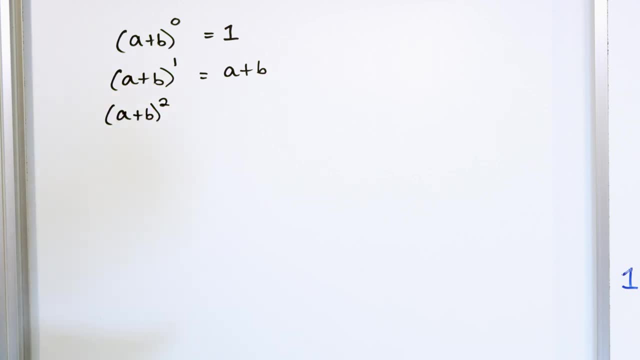 Now I know that a lot of you know the shortcut tricks and memorize how to do that, but if you did it manually, what you would say is a plus b multiplied by a plus b. That's what this means, right. 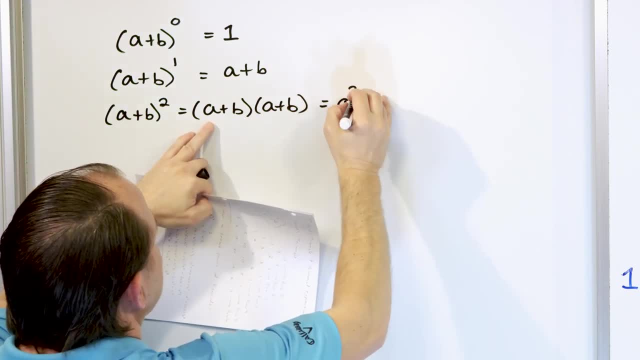 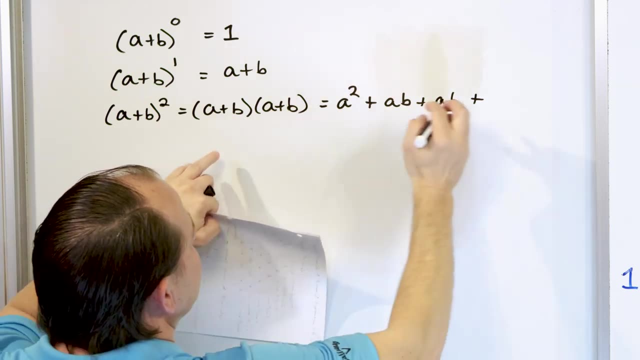 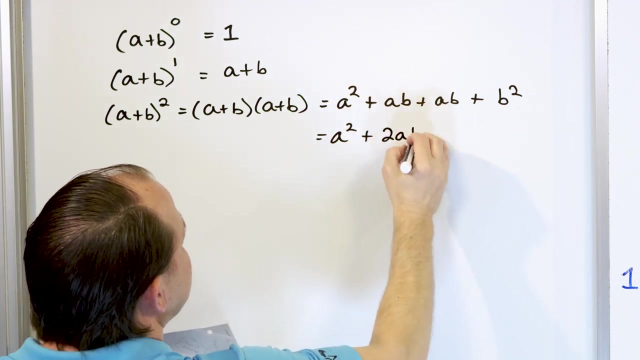 And how would you multiply it out? You would say: first terms: a squared, inside terms is a, b, outside terms is also a, b and last terms is b squared. So when you multiply these together, you get a squared plus two here, times a, b plus b squared. 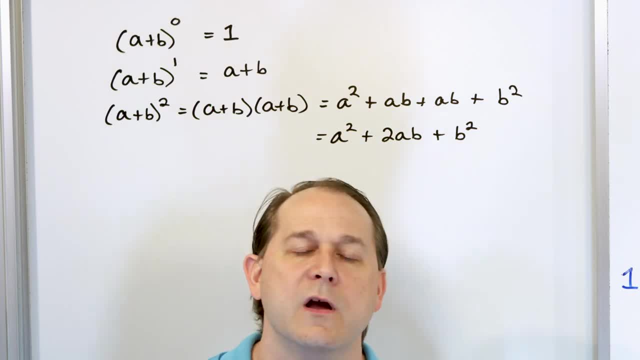 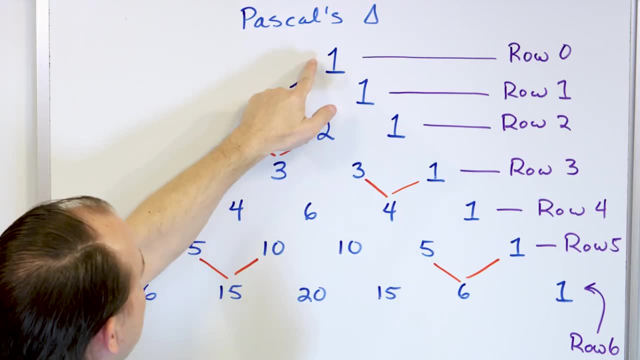 Now you might say: why do we care about this? Now I'm gonna do one more or I do anything else. Let me just point out to you something really quickly. Notice: Pascal's triangle has a one in the top. Notice the coefficient here in the answer is a one. 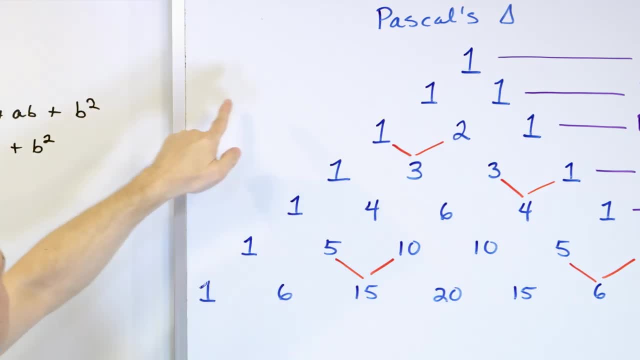 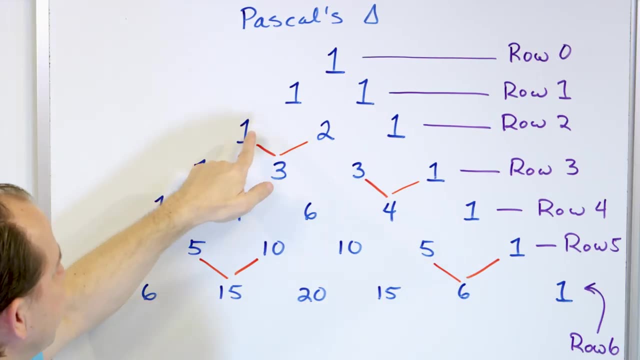 The second row of Pascal's triangle has a one and then a one. Those are the coefficients of this. There's a coefficient of one in front and a coefficient of one here- Notice- in row three of the triangle, that is one, then two, then one. 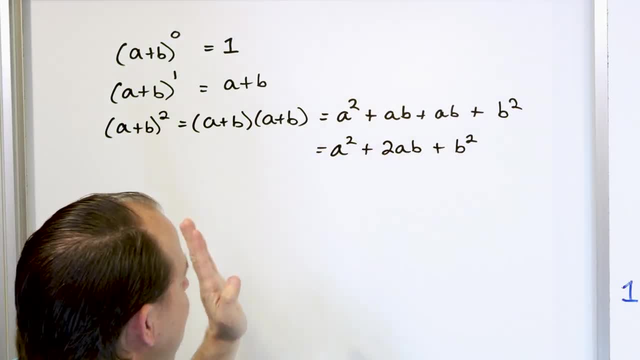 Notice, those are the coefficients: one, then two, then one. Now I understand that we have an a squared and an a squared and an a b and a b squared, and you're like: oh, it looks confusing. 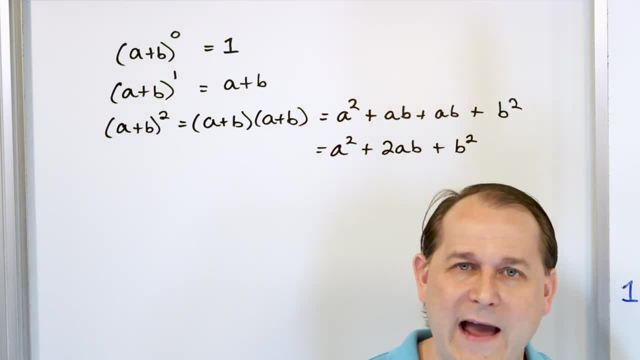 But all I want you to know right now is that it appears that the triangle predicts the coefficients that are gonna be in our answers as we keep making larger and larger powers of a plus b. So when we say binomial expansion, remember a binomial is just anything. 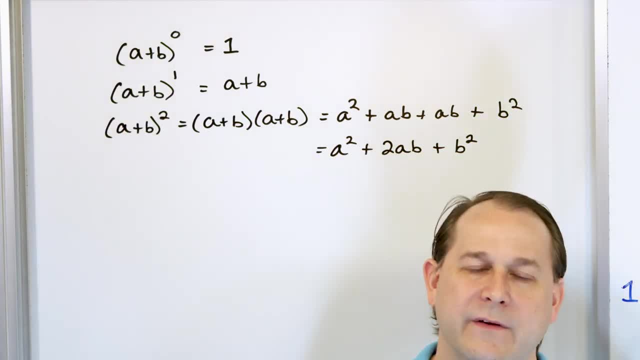 with two things added together: Bicycle means two wheels, So binomial means two little terms, So we're expanding them to a power, And so we can see the terms. the terms match up. Now let's do one more. I'm not gonna go down this whole triangle and prove it to you. 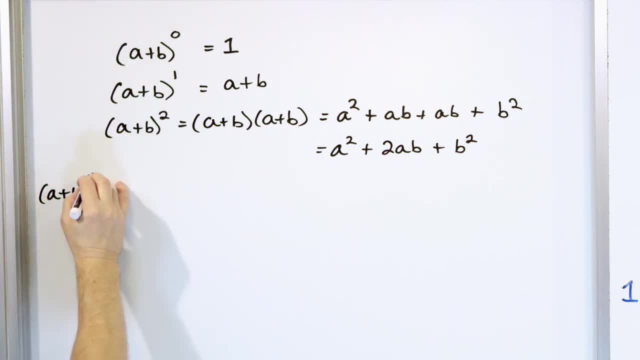 but let's do one more: a plus b to the power of three. How would you do this? We don't have a ready-made formula, but you know that this is the same as a plus b times a plus b squared. You know that because you can add the exponents. 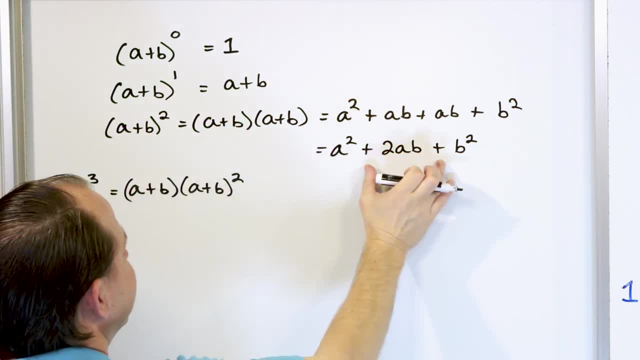 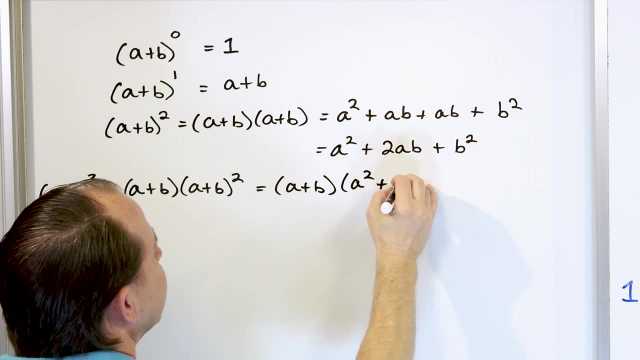 and get the three. But we just calculated what a plus b squared is. So really this is a plus b times what we just arrived at: a squared plus two a squared, Two a b plus b squared. So this results. it reduces down to having to multiply this. 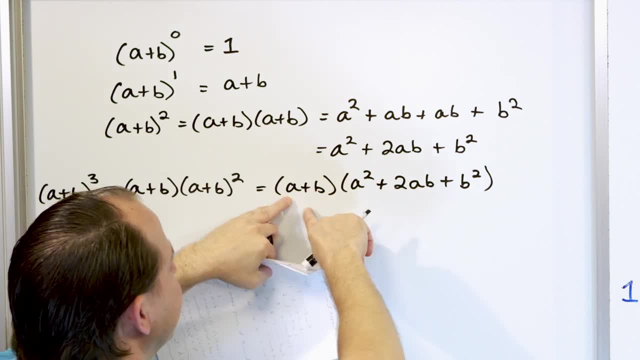 Now you can see where the pain comes from, because to do this multiplication, you'll distribute in, distribute in, distribute in the a, then you'll move to b, distribute b, b and b in. So let's do it real quick. 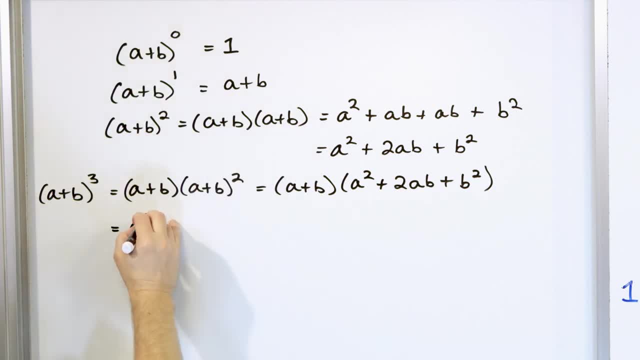 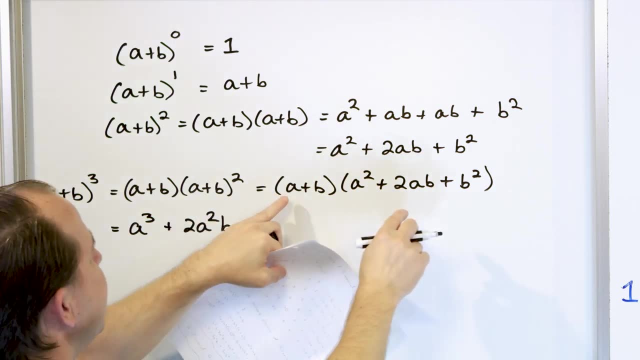 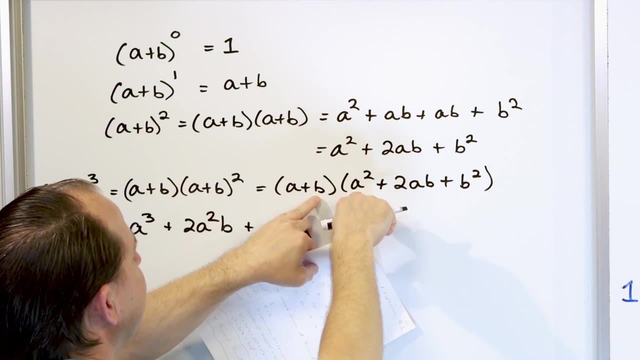 I think it's worth doing A times. a squared is a cubed A times. this is two times. then a squared b And then the a times. the third term is a, b squared. All right, now we move our finger to b and push it in. 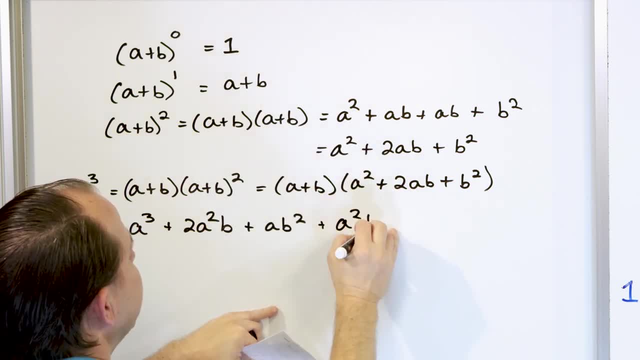 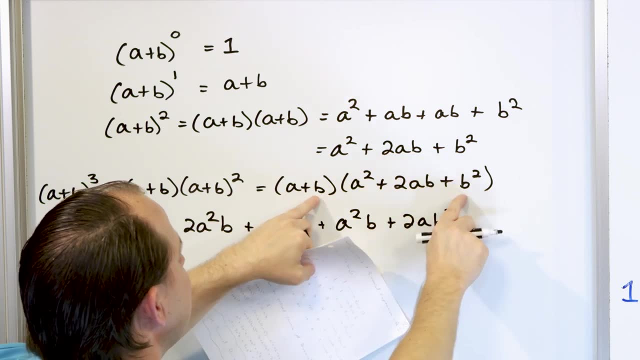 So it's gonna be b a squared. We're gonna write it with the a term, first a squared b, Then b times. this will be two a- b squared, Two a- b squared, Then the b times. the b squared will be b cubed. 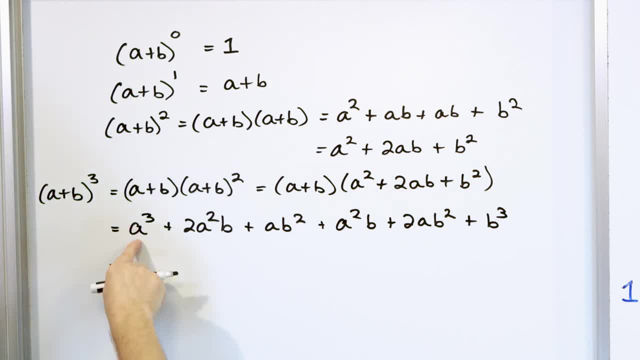 See how many terms I have. It's really ugly, But I have. I can combine some of them. So I have a cubed Notice, I have two a squared b and then I have an a squared b here, So I have another one of those. 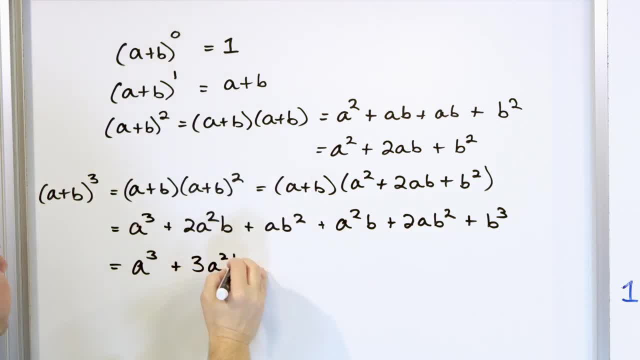 So I can add those together and make it three times a squared, b. So I've added that Now I have a, b squared and I have a, two, a, b squared, So I can add that for a, three, a, b squared. So I've really taken care of all of these terms. 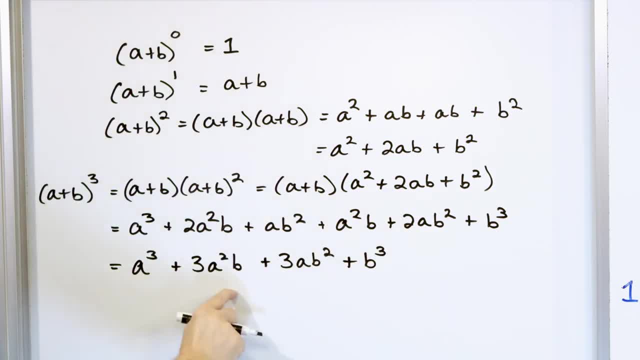 The only thing left I have is this one b cubed. So this is equal to a plus b raised to the third power. So, if our theory is correct, the coefficient in front of here, in front of here, in front of here and in front of here should be one three. 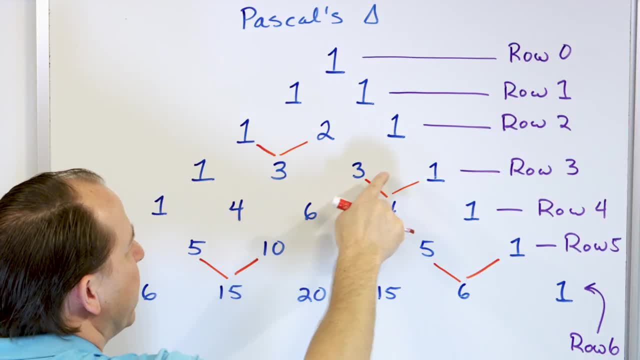 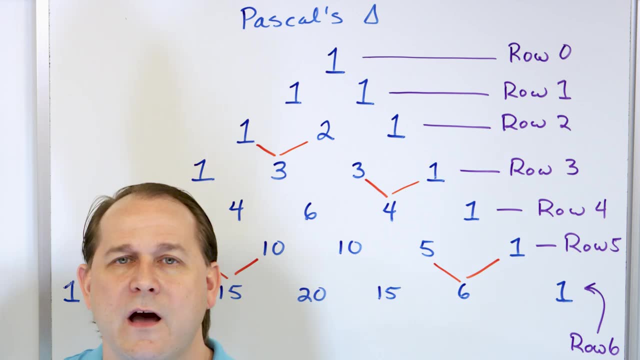 three, one. The next row of the triangle is one, three, three, one. So I'm not going to go any farther, but I hope that I've proven to you that this Pascal's triangle actually does predict the coefficients of all of the answers. 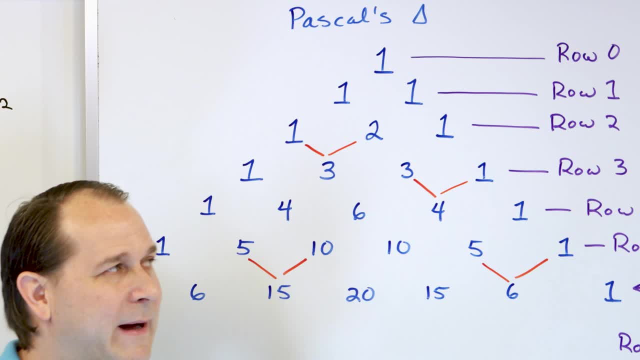 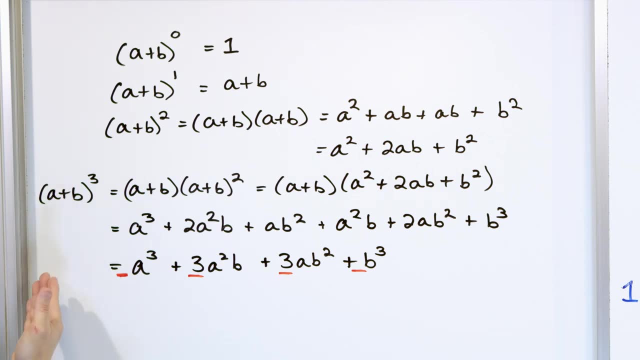 of what we call binomial expansion. So if you need to expand the binomial, like in this case, we've done a plus b to the first, a plus b to the second, a plus b to the third. If you needed to do, for instance, 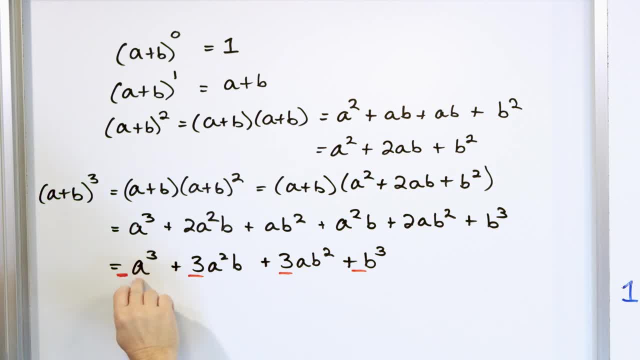 a plus b to the fourth power, then I'm going to show you in a second how to get all of these a, bs and stuff together. I'm going to show you how to do that. But the coefficients themselves of a plus b to the fourth power must be one, then four. 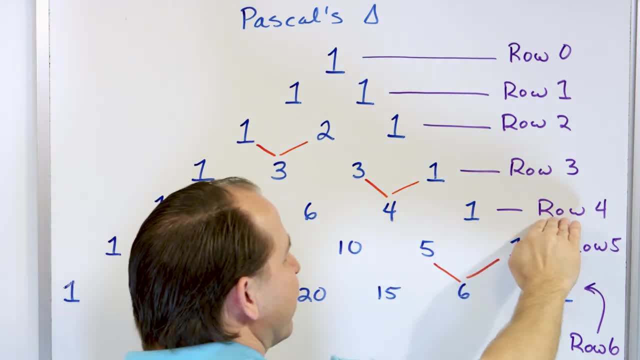 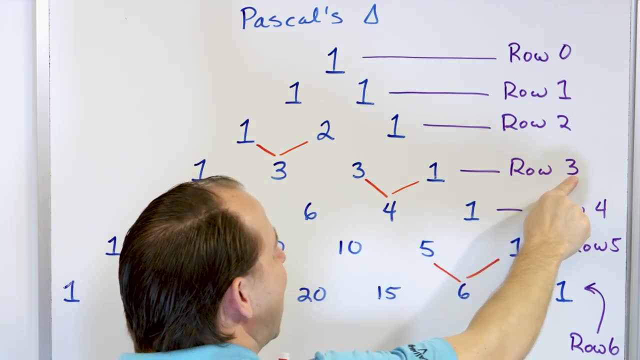 then six, then four, then one. That's why I labeled this row four, because a plus b to the fourth power. you just look at row four and there you go: A plus b to the third power. you read this line off. 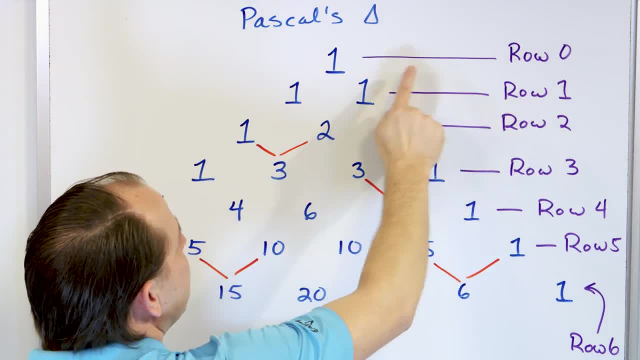 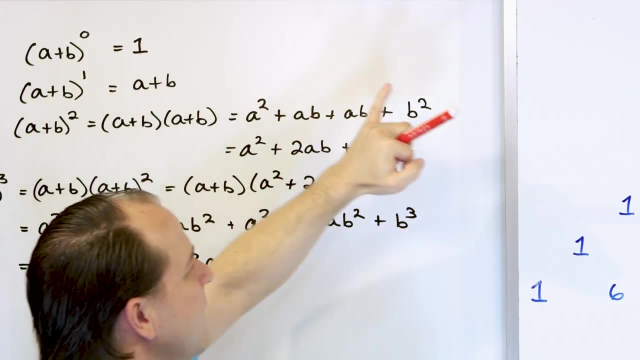 A plus b to the second power, this one to the first power, this one. And now you know why this is labeled row zero: because when you take a plus b to the zero power, that gives you one, which is the top of the triangle. 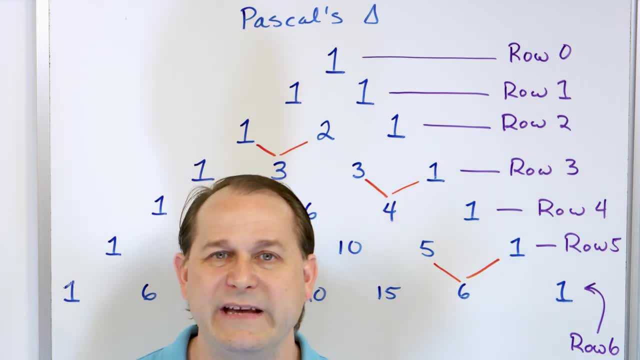 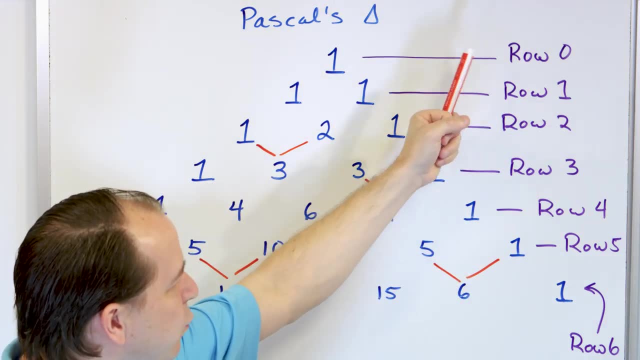 So if we were to label this row one, it would get confusing. but it's very easy now. If you're just expanding a plus b to the- let's say, the sixth power and you label row zero, then one, two, three, four, five. 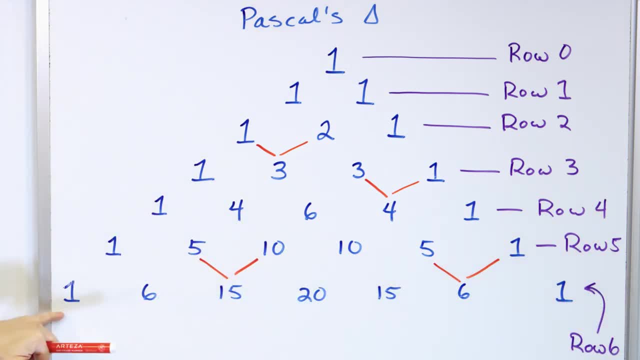 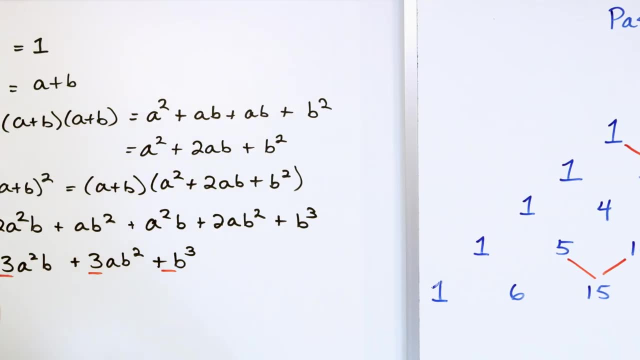 one more row down here is six, then a plus b to the sixth, power is going to have all of these coefficients in the answer. All right. so what I want you to do is take a look at what we have here and try to keep them in your mind. 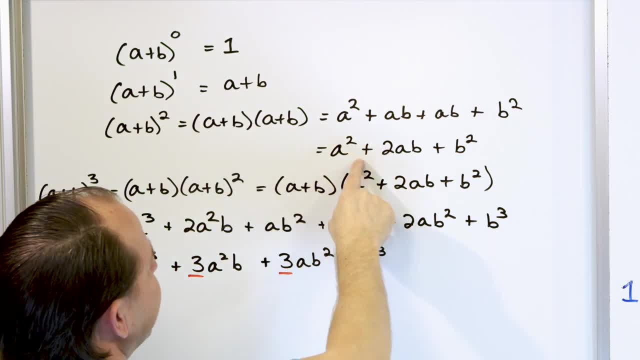 First we had a one, then we had an a plus b, then we had an a plus b, then we had an a plus b, then we had a squared plus do a b plus b squared. then we had this large answer with the one, three, three, one. 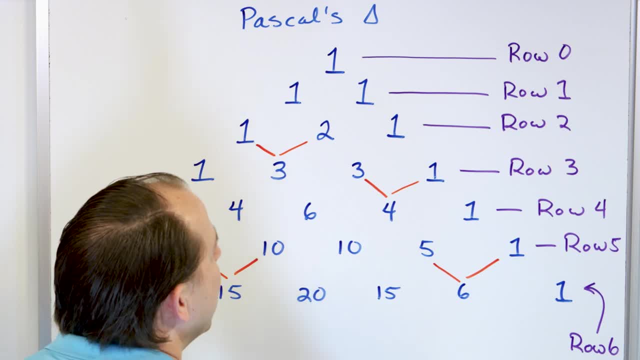 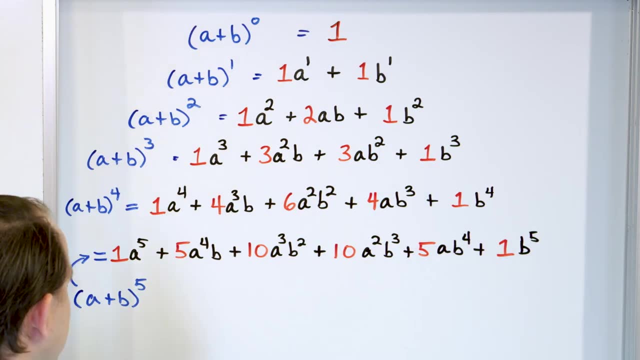 I've actually filled out a similar table to this on the next board already ahead of time. I just didn't want to hit you over the head with it. This is the first six, actually the first: zero, one, two, three, four, five. 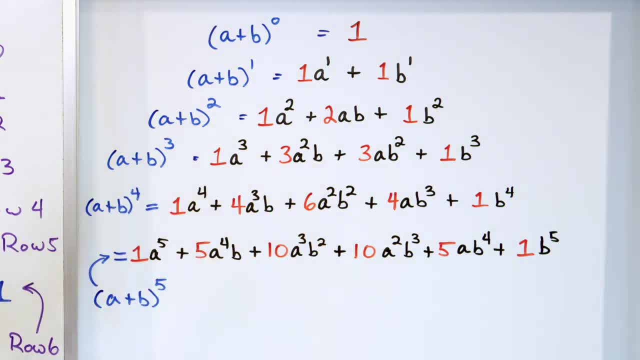 yeah, the first six levels of Pascal's triangle here actually the first one, two, three, four, five, yeah, six, I don't know how many of them lines here, And so what I've done is I've kind of tabulated it here. 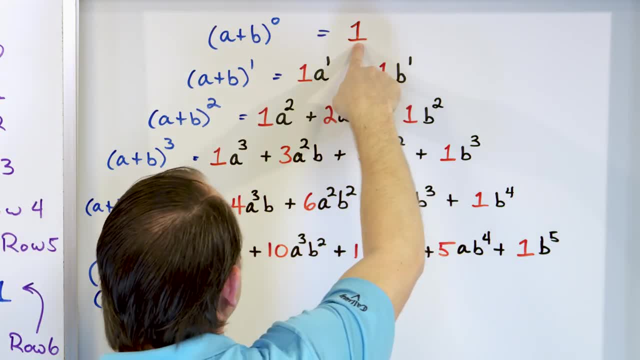 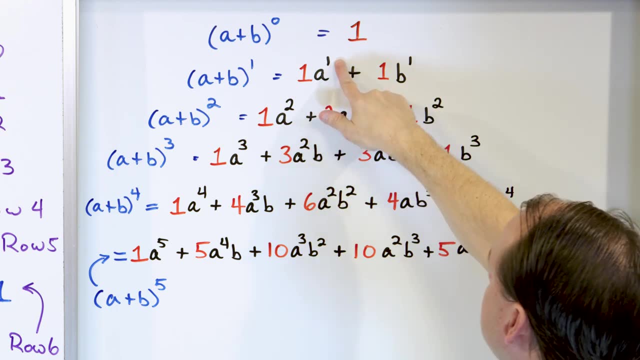 So a plus b to the first. power is one, and I've colored the one in because this is going to now match Pascal's triangle with that one. Then you have a plus b to the first. It's one a to the first plus b to the first. 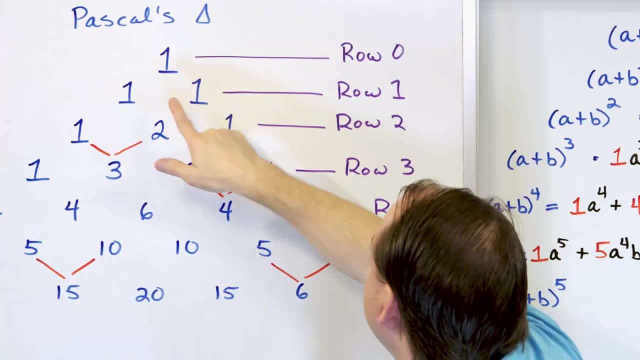 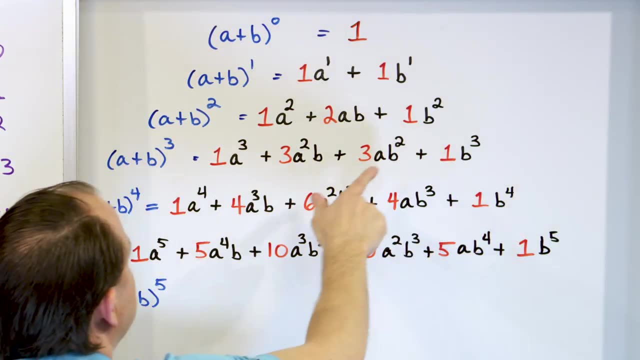 or you can think of it as just a plus b. The one and the one come straight out of the table and you can just read it down: One, two, one come from there. Then we already did one, three, three, one. 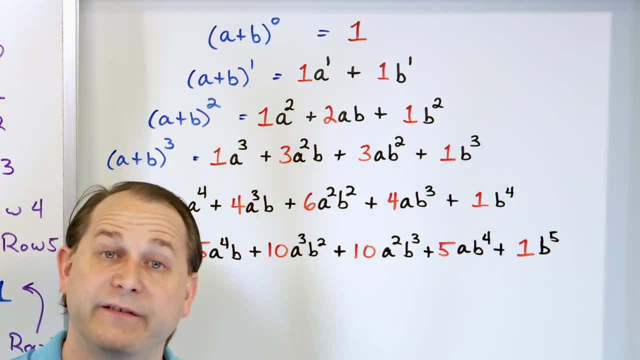 comes straight out of there. If you were to continue multiplying a plus b to the fourth power, you'd have a ton of things to multiply and add together, but you would arrive at this And it would be one a to the fourth, four a third b and so on. 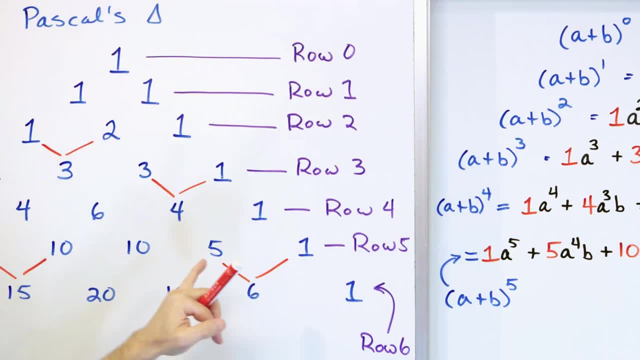 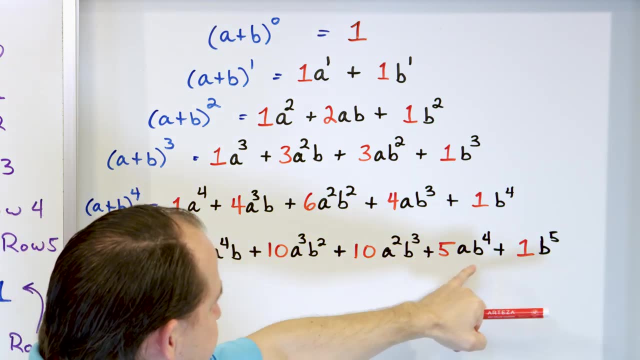 But the coefficients one, four, six, four, one exactly match the table. And then again a plus b to the fifth power: one, five, 10,, 10,, five, one match this. One, five, 10,, 10,, five, one. 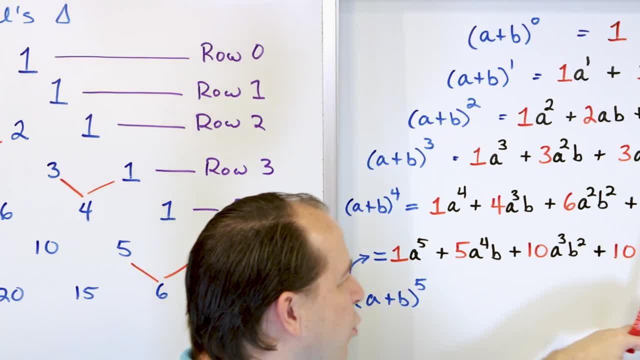 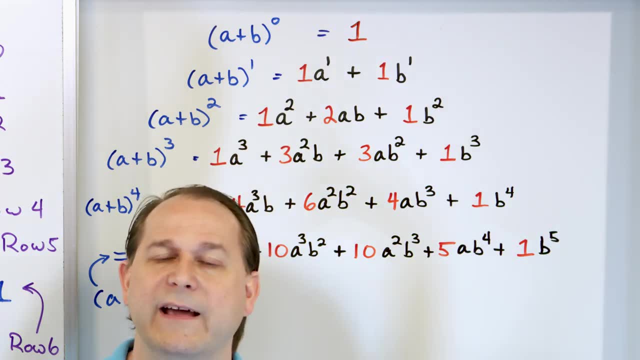 Now I took this table one more row and I didn't bother to write one more row here because I'd be writing forever. So I just wanted to show you that when you expand these binomials, it does form a triangle that can be predicted exactly from Pascal's triangle. 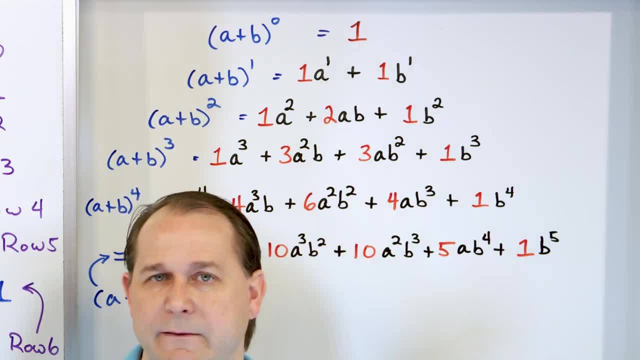 So it allows you to do something like a plus b to the 17th power, as long as you know the elements of that triangle. all right, Now I have to give you a couple notes here before we do any problems, because ultimately, the problems I wanna give you, 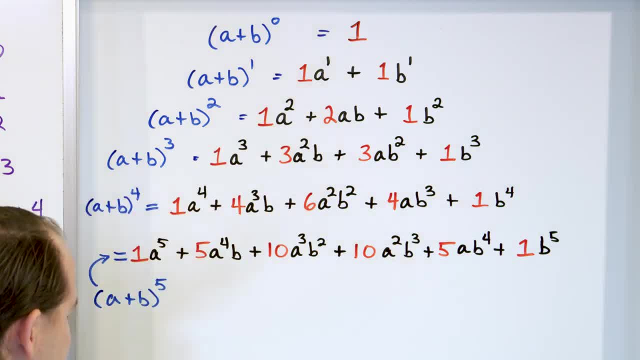 is: I want you to expand binomials, right? So I need to show you some really important things, okay? The first thing is: you may not have noticed before, but now, when they're all on the same board, look at a plus b to the power of two. 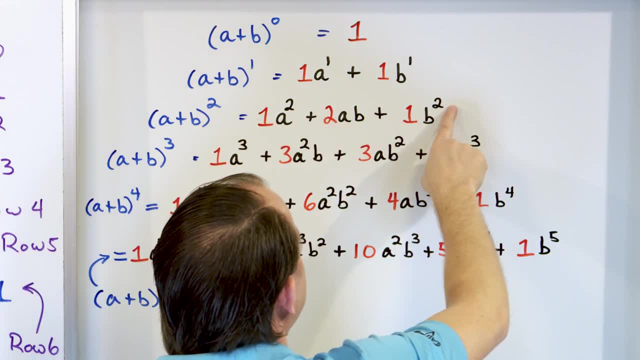 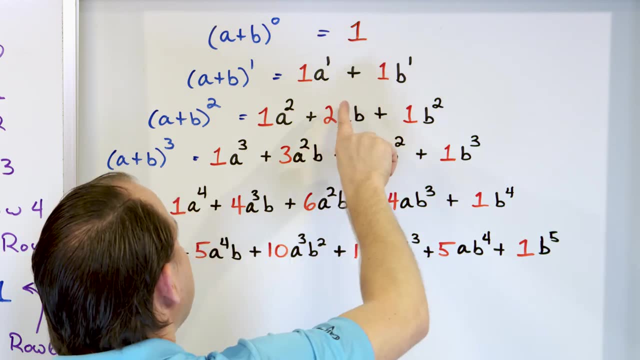 Notice that this is a? squared and the last term is b? squared and the middle term is just a times b. but a has a power of one and b has a power of one. If you, in your mind, add one plus one, you get two. 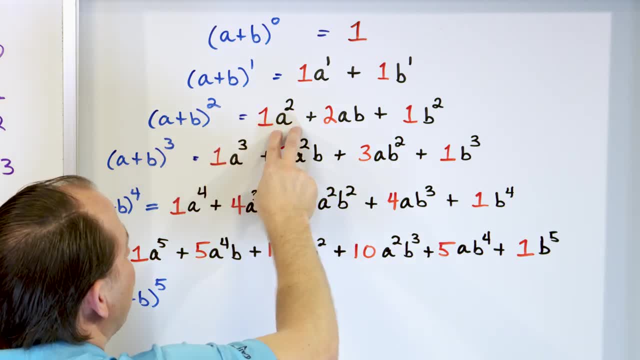 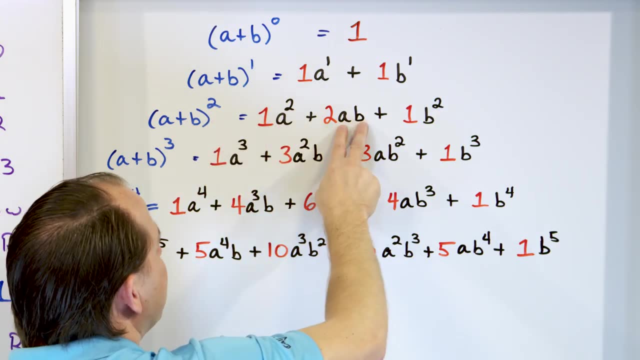 So really, when you're taking a plus b and you're squaring it every term, the sum of the exponents must be equal to, in this case, two. Notice the exponents add to two. The exponents here add to two. 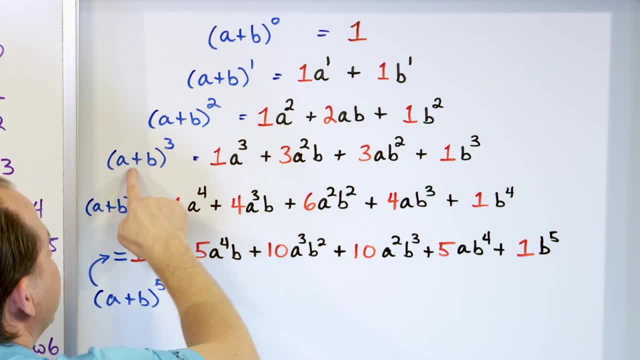 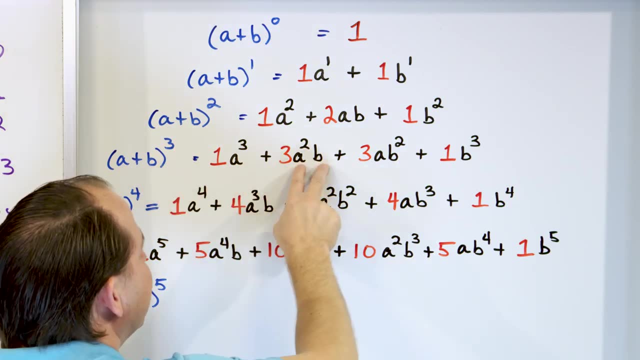 The exponents here add to two. okay, Try it for the next slide. This is a plus b cubed, So this is a cubed. so the exponents add to three. matching this. These exponents add to three. These exponents add to three. 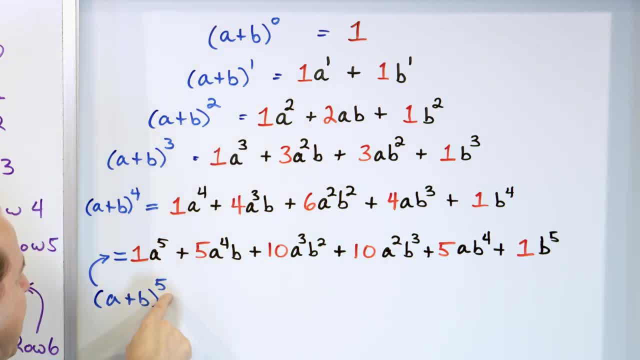 These exponents add to three. It's the same pattern for all of it. If you look at a plus b to the fifth, every exponent, in every one of these terms, they must sum up to the power of the thing you're expanding to. 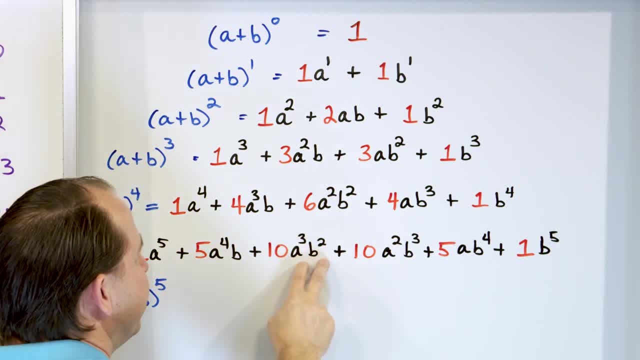 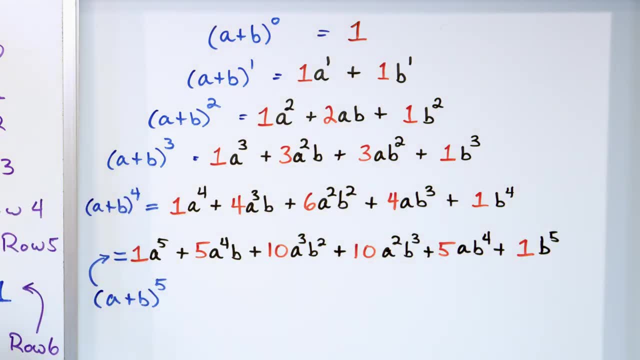 So the sum of these exponents must be five, must be five, must be five. Three plus two must be five, Two plus three must be five, One plus four, and then must be five b to the fifth. So the trick is, if I just asked you, 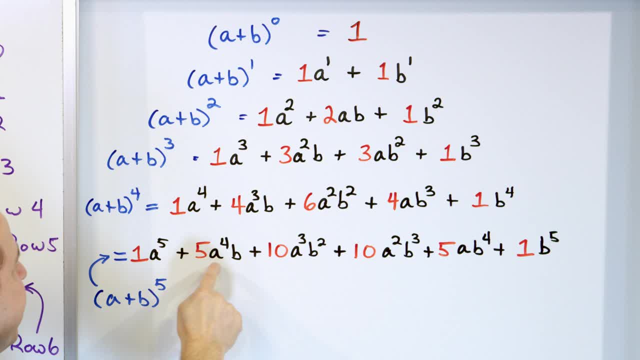 tell me what a plus b to the five is. the first thing you need to know is what these coefficients are. You can get those just by having your Pascal's triangle written down on paper. The second thing is you need to know- I'm talking about doing this without multiplying it all out- 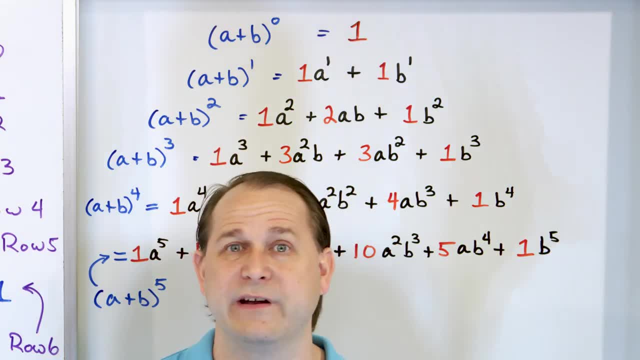 You saw how much of a pain it was just for the cube. Imagine if you did it for a sixth power. It would have numbers and letters everywhere. So you have to know the coefficients. That comes from Pascal's triangle. How do you predict all of these little terms here? 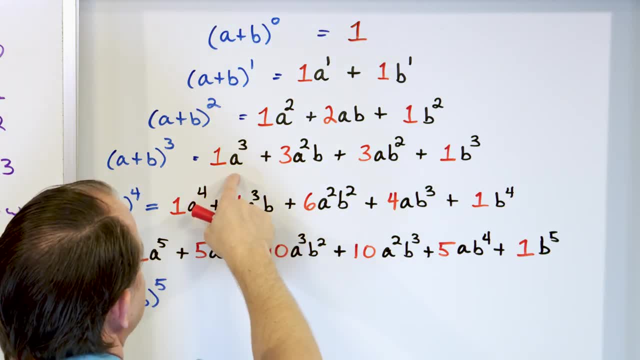 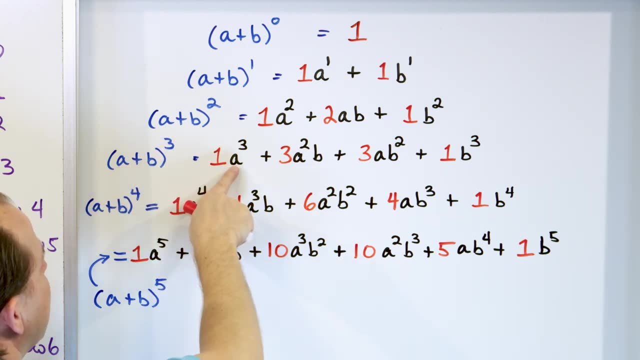 Let me show you a little secret. Let's go look at this one, for instance- This is probably the easiest one to look at- To the cube power. what you do for the first term is you start with a cubed just by itself. 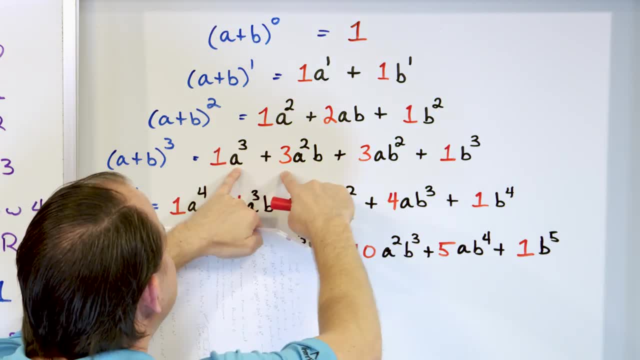 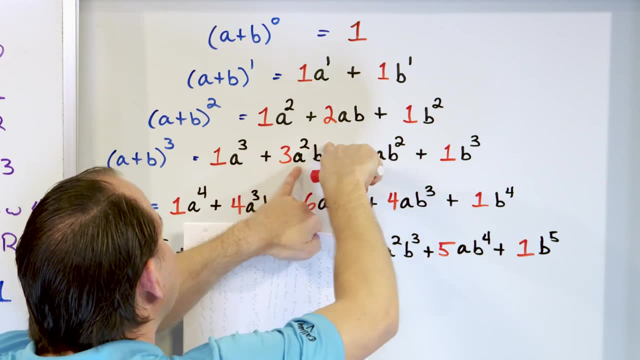 Then, for the next term, what you do is you're always reducing a down by one. So notice: this is a two. But in order to make it all equal, three b has to come up from a zero power. it has to come up to a one power. 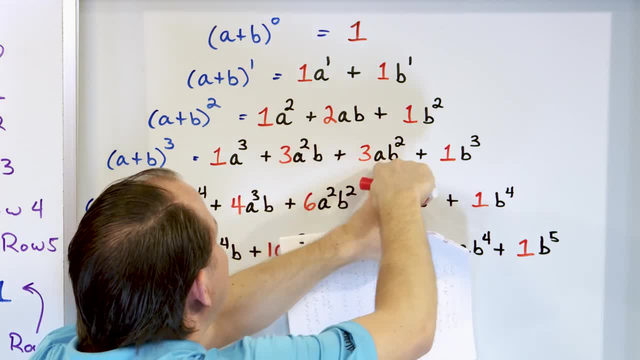 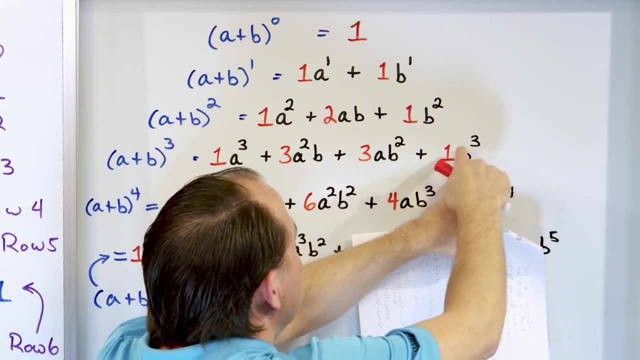 So b goes up a power, In the next term a again goes down a power and b then goes up a power, And then in the last term b goes down a power to a to zero, which means it's one, it disappears. 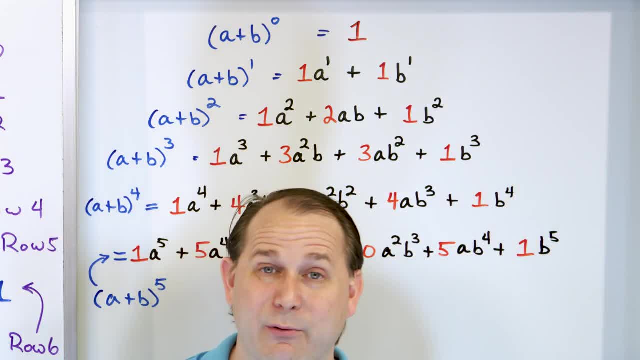 and b goes up. a power. This pattern is really powerful. It allows you to predict any binomial expansion you want to. All you do is you start. let's go with the next one. You start with a to the fourth. that's the first term. 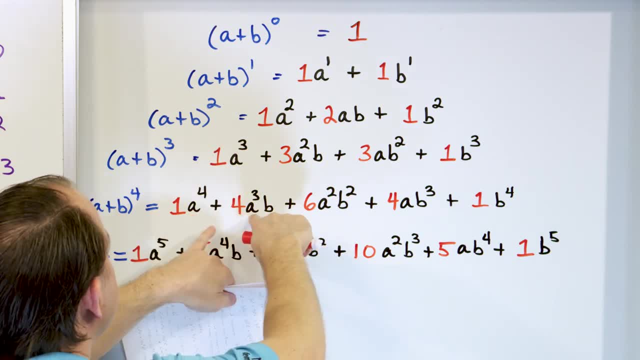 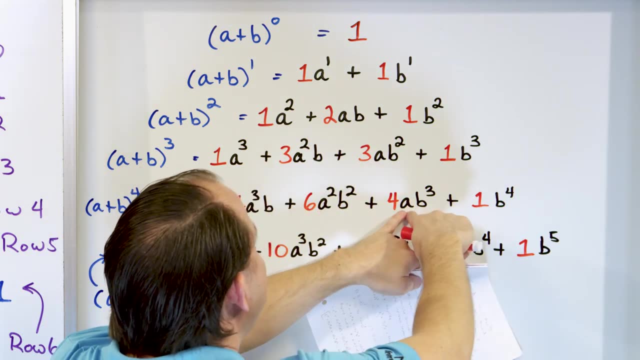 Then to write the terms down. all you do is you make a go down by a, power b goes up. Then you go down here: a goes down by another, power, b goes up. Then you say: a goes down by a power from that one, b goes up. 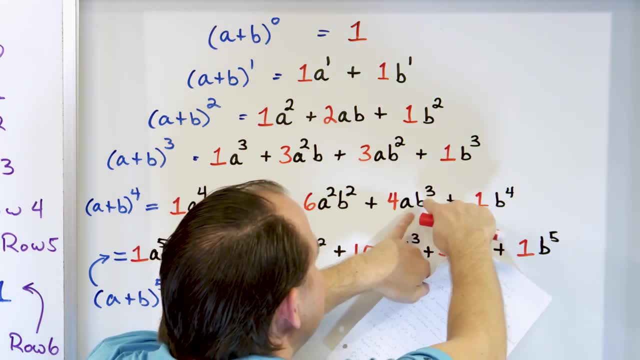 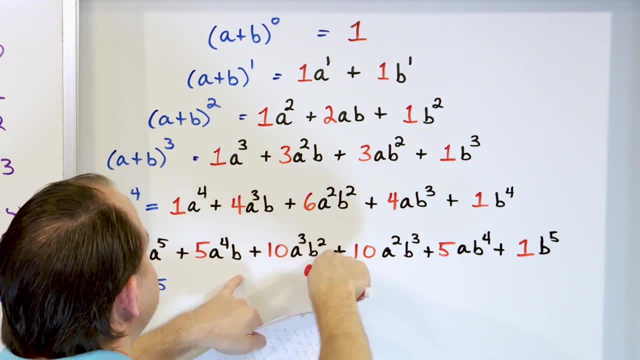 a goes down by a power to a to the zero, which means it disappears, and then b goes up. Same thing is happening here. You say a to the fifth is your first one. a goes down, b goes up. a goes down, b goes up. 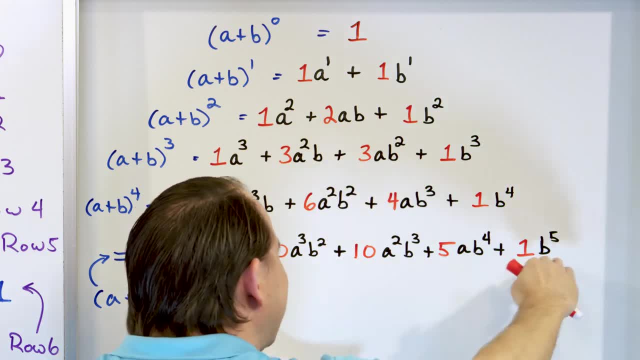 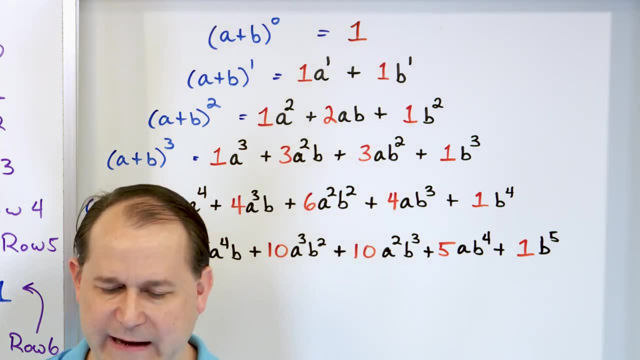 a goes down, b goes up, and so on. a goes down, b goes up all the way to the end, And then the coefficients in front of all of those terms just come from the triangle. So let me make sure I have everything I have in my notes. 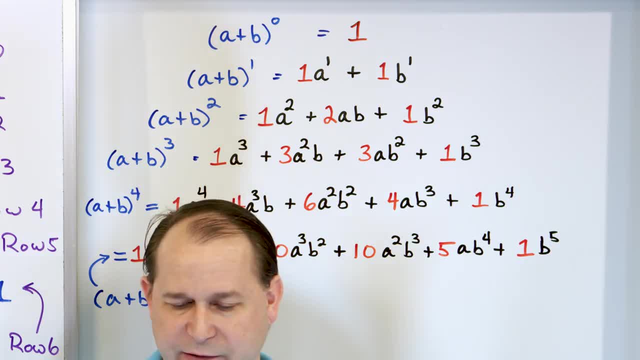 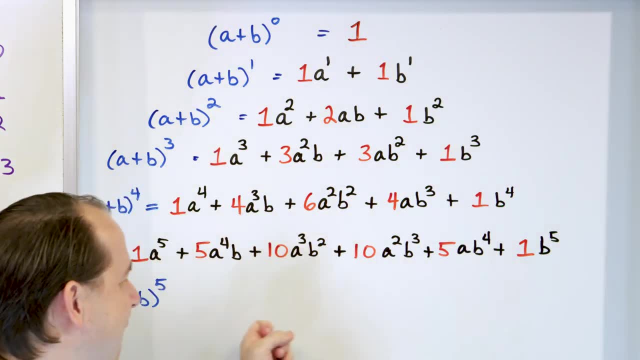 here Some of the exponents power, the binomial Coefficients are from Pascal's triangle. And then, as one of the variables decreases, the other one increases in such a way that they always add up to the power that you are expanding to. OK. 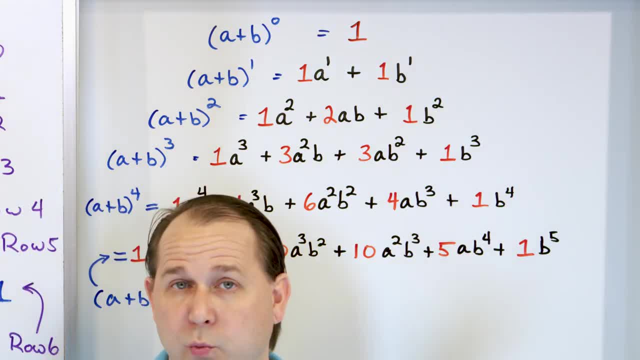 So by knowing this, you can write down an expansion of any binomial you want. The only limitation is that you have to know the numbers in this triangle. So if you're going up to a sixth power, I have it written for you here. 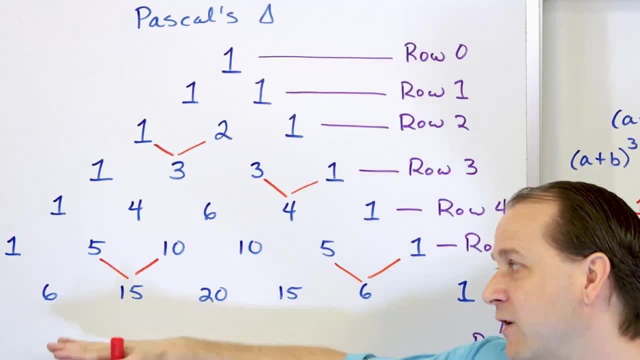 But if you need a seventh power, or an eighth power, or a ninth power, Or a tenth power, you're going to have to fill this triangle out even deeper than I have here. All right, So what I want to do now, I think 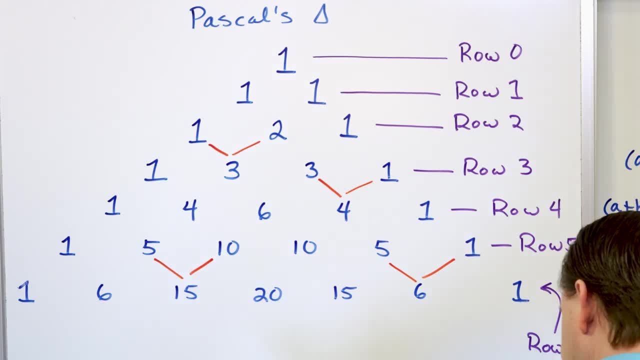 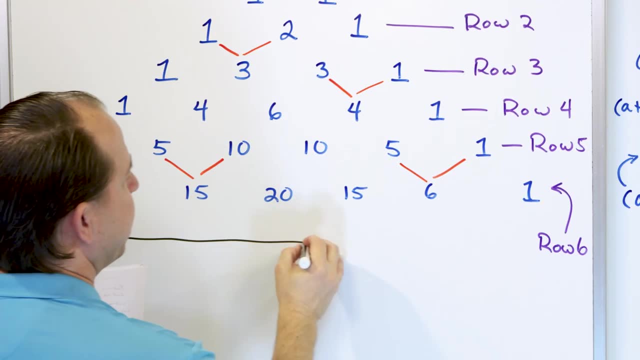 is solve a couple of problems. All right, I think I can do. let's see here. Yeah, I think I'm going to do a couple of them right underneath this Pascal's triangle, Because they're very simple and they powerfully. 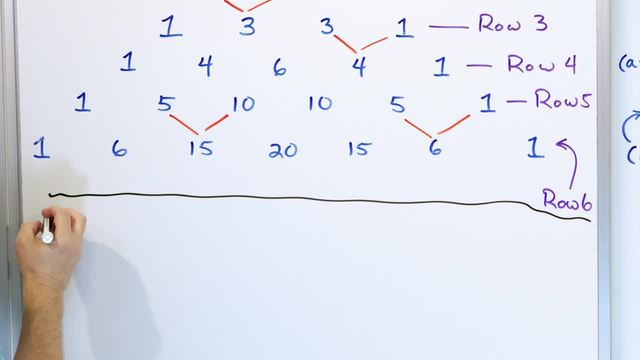 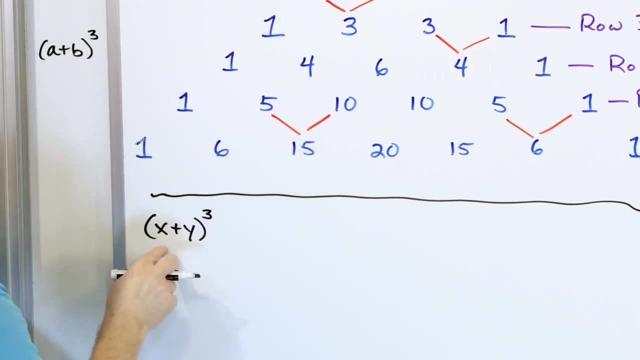 illustrate how to do this. So let's do the first one. Let's just go ahead and write down x plus y to the power of 3.. Now the way we did this before is we actually did the FOIL, multiplied it all out, added all the terms and we end up. 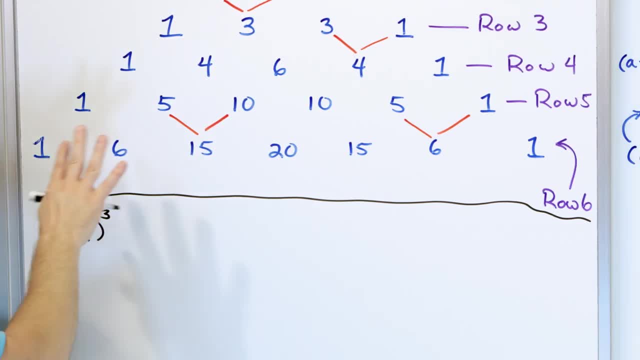 So we know what the answer is, But that's no fun. We want to do it using this more powerful method. Here's what you do. The first thing we need to do is say, OK, we're raising to the third power. 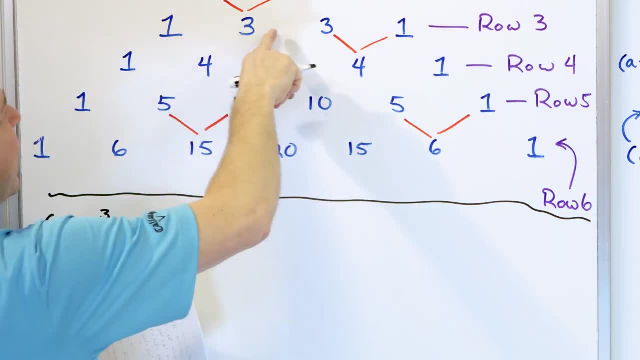 So we go to row 3 in the triangle. The numbers from this triangle are exactly written here: 1,, 3,, 3, 1.. So I recommend that you write in your paper: Pascal triangle: 1,, 3,, 3, 1.. 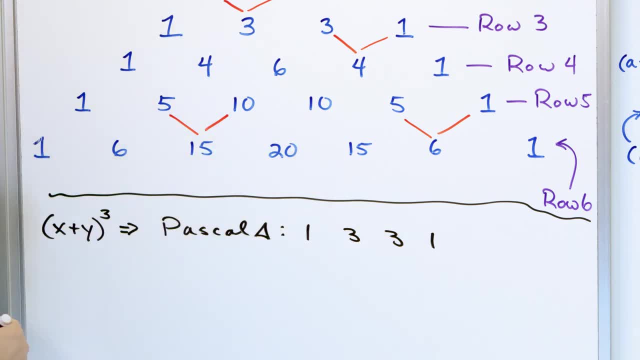 This tells me the numbers I have to use in the expansion of this thing, right here, Next, All right, So the first thing is just going to be the first term, the first thing in your binomial cubed with a coefficient of 1.. 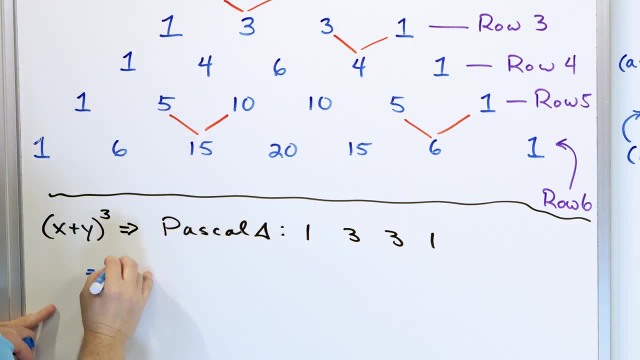 So I don't need to write a 1 down. I can just say it's going to equal x cubed, Because I have a 1 here. That's the first coefficient. Then I'm going to have a plus sign. The next term is going to have a coefficient of 3.. 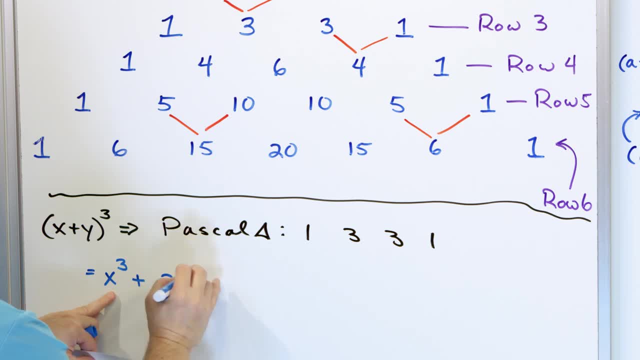 And then what do I do? I say x goes down a power, So it's going to be x to the power of 2.. And there's a y here. y has to go up a power. It was y to the 0 here, which means y to the 0 is 1.. 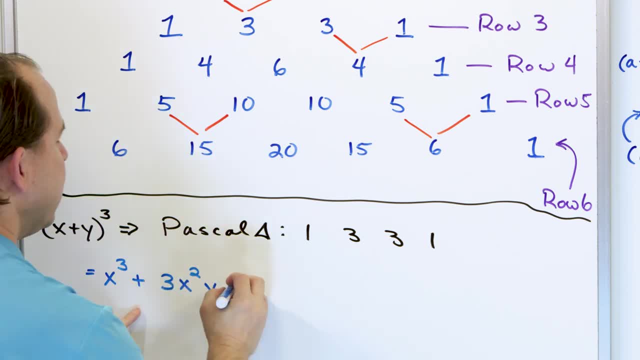 So it goes up a power just up to y, to the first power, Then the next term grabs the next 3. And then again, x goes down a power, x to the first power, And y then goes up a power, like this: 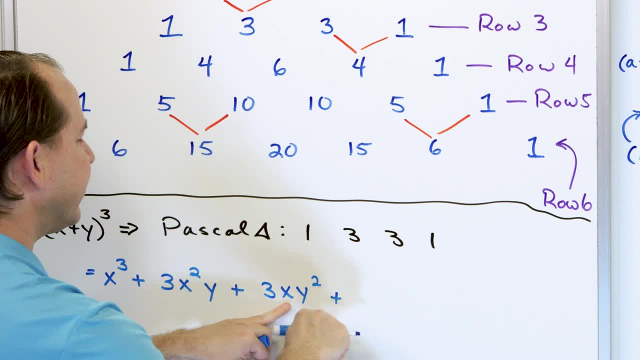 And then, for the last term, it's just 1 as the coefficient, And then again x goes down a power. So you could say x to the 0, making it just 1.. And then y to the third. So this is the answer. 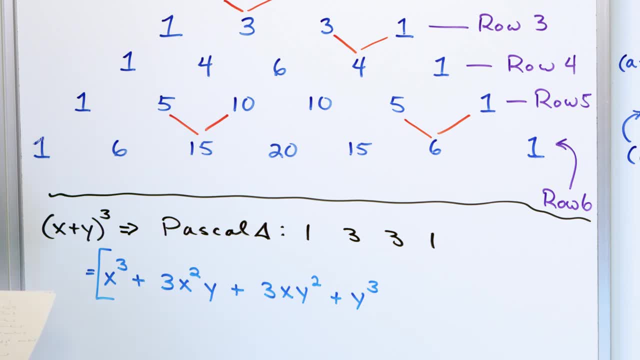 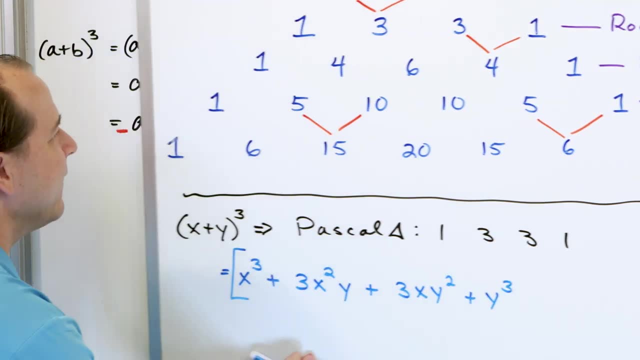 And notice- let me just double check- x cubed plus 3x squared y plus 3xy squared plus y cubed. Notice that I was able to write this down more or less without doing very much work and compare that to something like this: 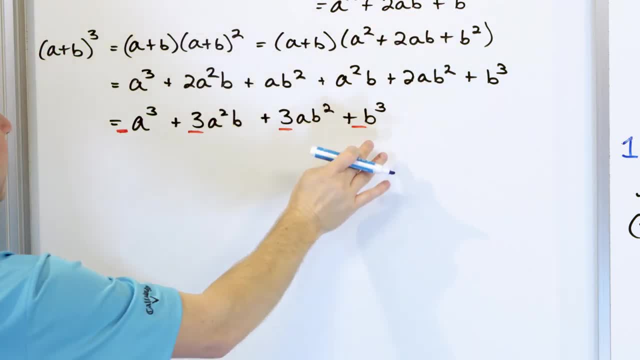 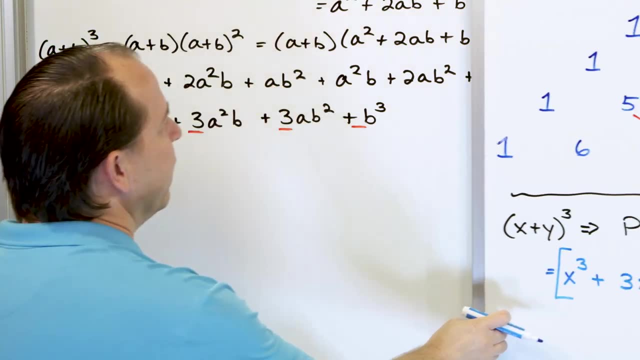 I had to first FOIL this, then cross, multiply everything in, then add the terms and then really hope and pray that I didn't make an error, because it's really easy to make errors. All of us make errors. I make errors all the time. 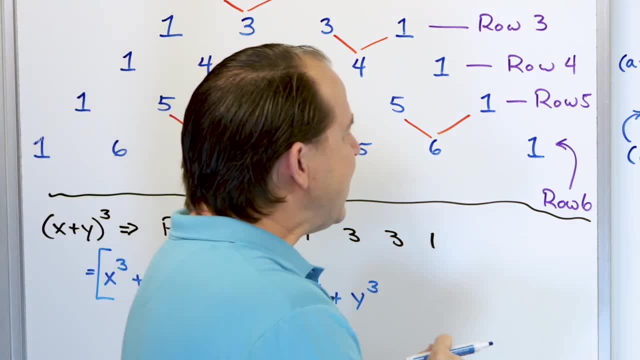 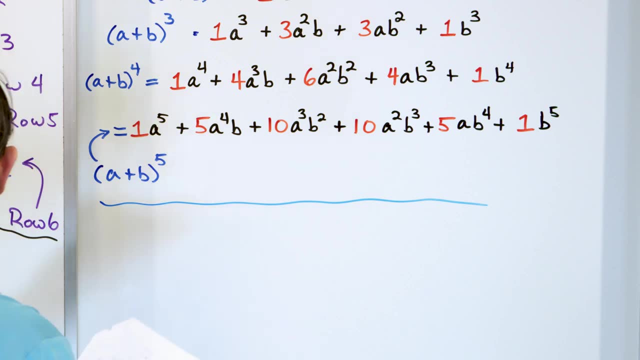 And so it can just happen. So that's how we do it. Now what I want to do is just do a few more, just to give you a little practice. What if I give you something a little bit more challenging than this? It's just x plus y to the third power. 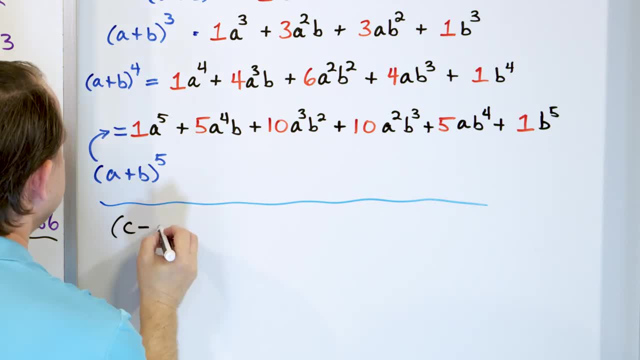 Now let's do one a little bit different. What if you do c minus d raised to the fifth power? A couple of things. that makes it difficult. You have a fifth power, So I'm going to be using the row number 5 of the Pascal's. 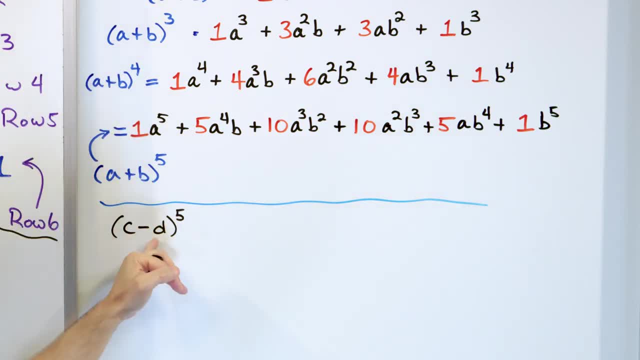 triangle, But also there's a minus sign in here, And also we're using c And d. This is what I want you to do Any time you have anything other than a and b in there. this is what I want you to do. 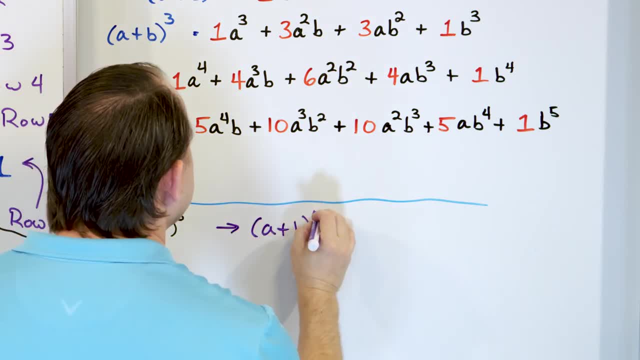 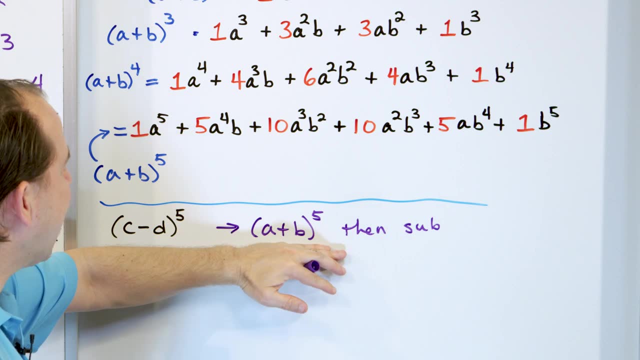 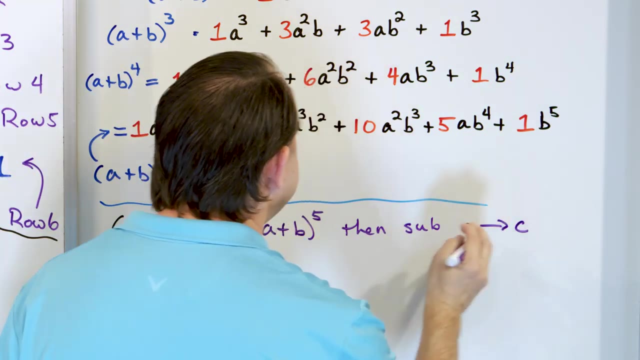 I want you to work on a plus b to the fifth power. then sub What I mean by that is, if you know it's to the fifth power, just expand a plus b to the fifth power And once you have the answer, then substitute: a goes to c. 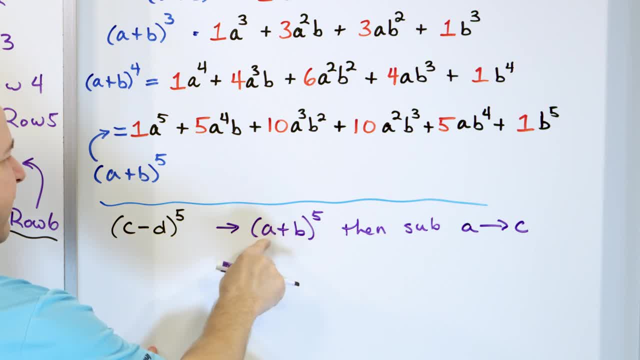 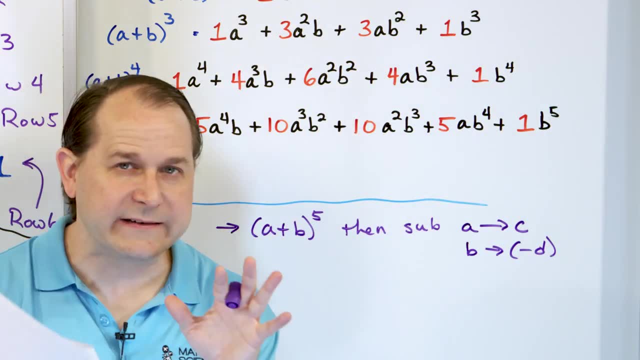 And then b here. once I get the answer in terms of a and b, I'll just I'll put negative d in for that. So I'll say b goes to negative d. So instead of trying to do too many things at once, which? 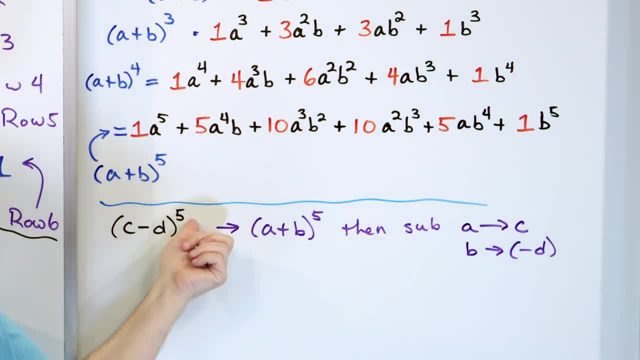 you will almost certainly make an error- just say: OK, I'm raising to the fifth power, I'm going to expand this. I know how to expand this very easily. Once I get the answer, I'll just substitute for a and make it this, and substitute for b and make it negative d. 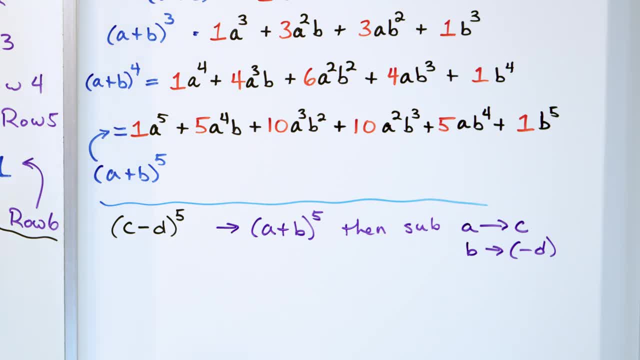 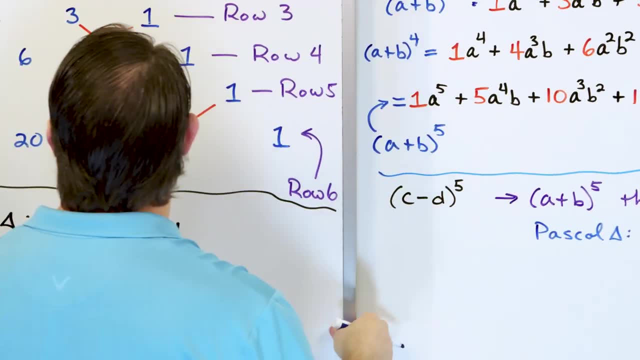 And then that will be my final answer. That's exactly what I'm going to do. And then I'm going to say: Pascal's triangle, what are the coefficients? So I go over here to Pascal's triangle. It's a fifth power of 5.. 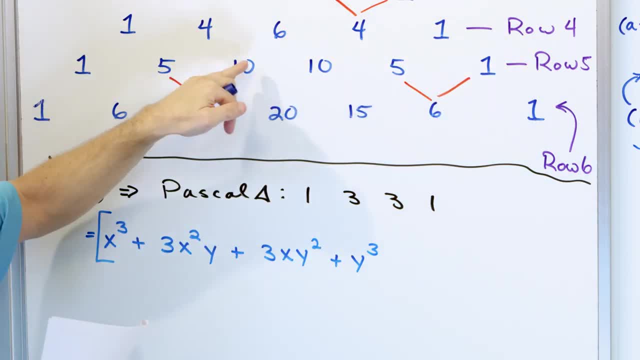 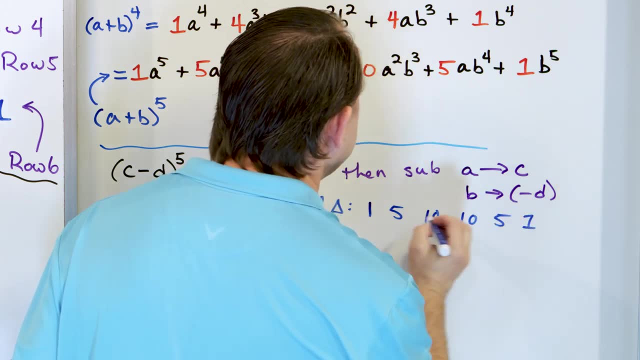 So it's row number 5.. So the numbers I use are 1, 5, 10, 10, 5, 1.. 1, 5, 10, 10, 5, 1.. 1, 5, 10, 10, 5, 1.. 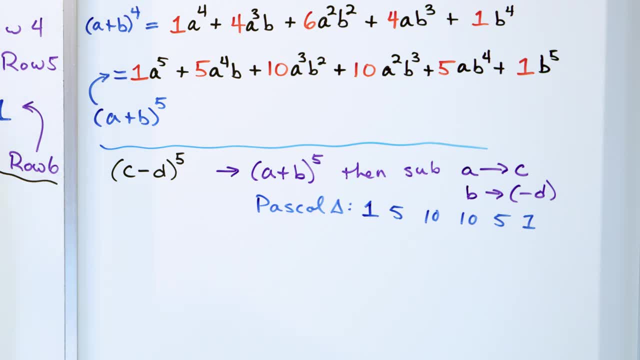 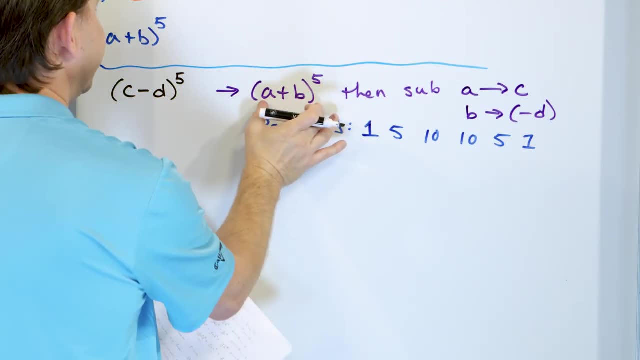 All I need to do is write them down on my paper so that I have some reference when I'm solving the problem, to actually use it. Now, what do we do? We're no longer working with this. We're working with this. What is the first term? 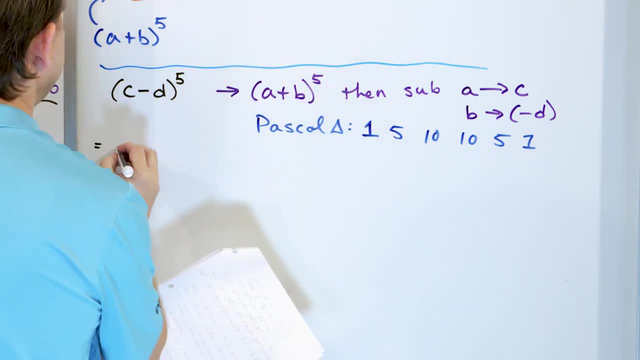 It's a coefficient of 1 a to the fifth. So we see, we just say a to the fifth. The next coefficient is 5.. So we put a 5.. Now what happens? a has to drop down by a power and b goes up by a power. 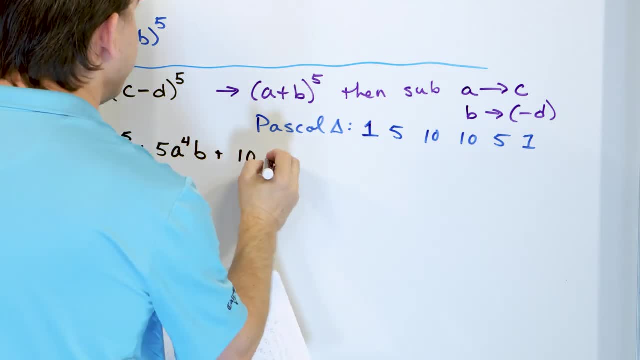 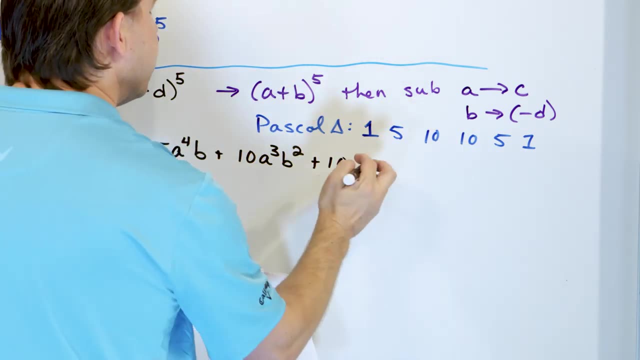 Next coefficient is 10.. a drops down by a power. b goes up by a power. Next coefficient, after this again, is 10.. a goes down by a power, making it a squared. b goes up by a power making it to the third. 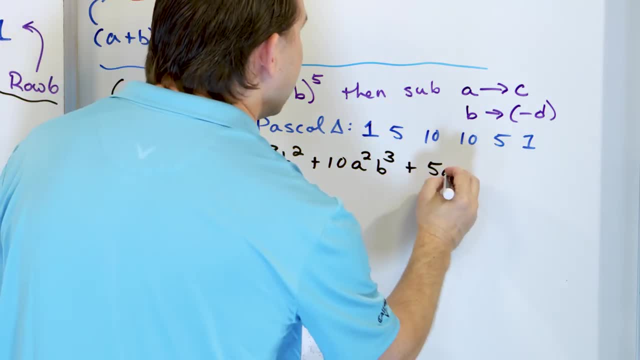 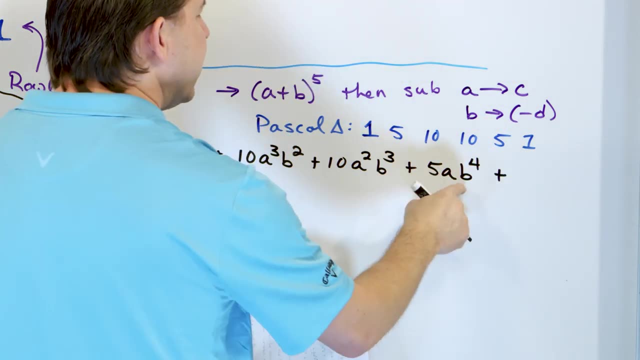 Next coefficient is 5.. a drops down by a power making it a to the first. b goes up by a power making it b to the fourth, And then the final guy is just a 1.. And then we drop a down to a to 0,, which means it disappears. 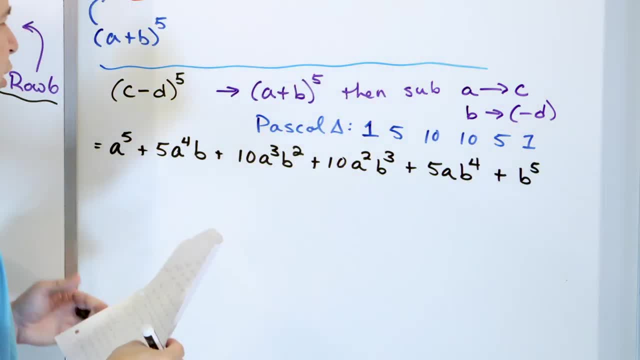 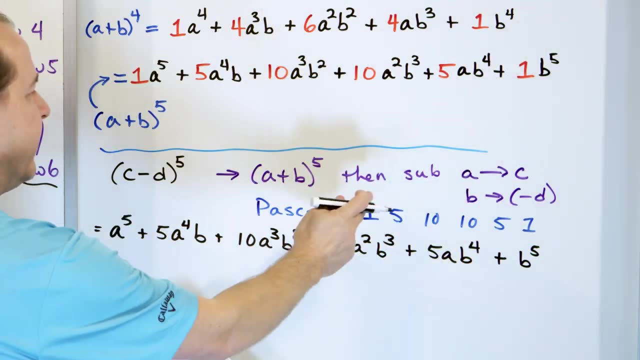 b goes up to b to the fifth, And the coefficient is 1.. It's a good idea at this step, all of these terms should have exponents that add together to give me 5, because I'm raising this thing to the fifth power. 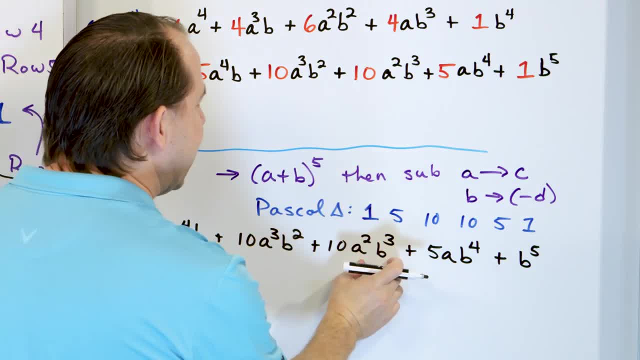 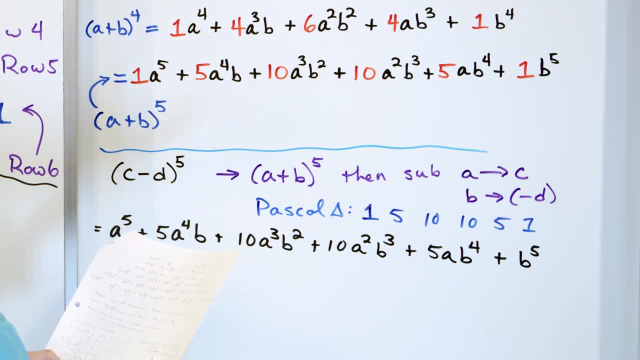 10a cubed b, 10a squared b, cubed. 5ab to the fourth, and so on b to the fifth. All right, so the next thing I need to do is I need to, everywhere I see an a. 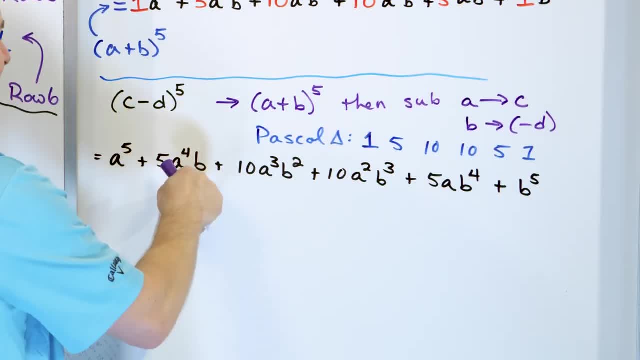 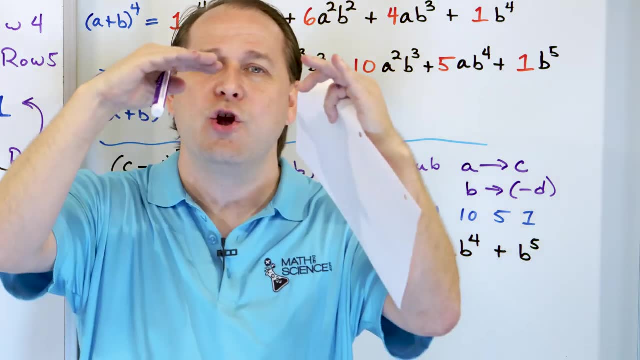 I'm just going to put the letter c in there. Everywhere I see a, b, I'm going to put a negative d, But I'm going to tell you right now, when you're substituting for b with that negative d that you want to put there, wrap it in parentheses. 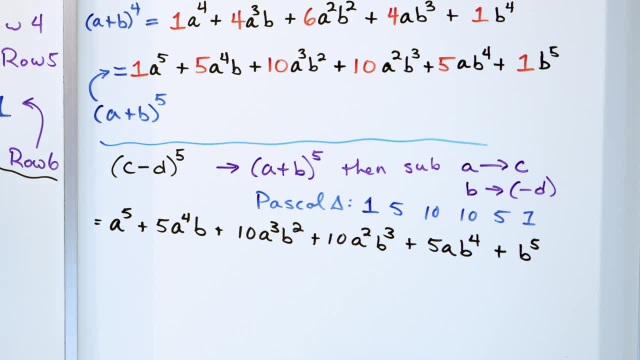 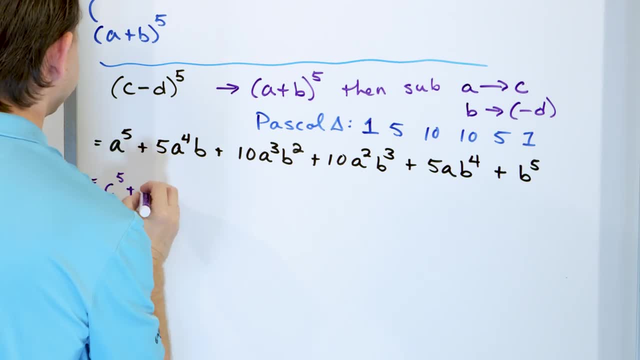 or else you're going to make a sign error somewhere. I virtually guarantee it. So a becomes c. So a becomes c. So what I'm going to say here, this is c to the fifth plus 5c to the fourth. 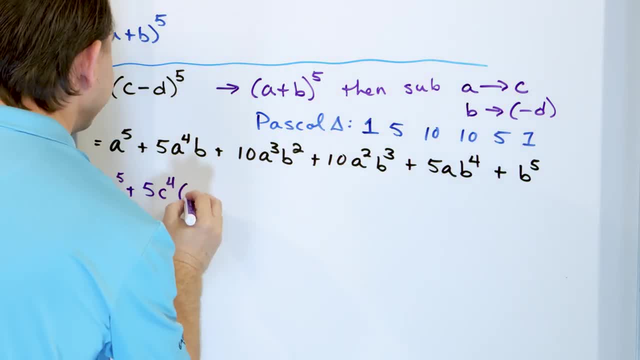 But I have a b. But b means I'm putting in negative d. Open a. parentheses make it negative d to the first power, so I don't have to really write a power there. I'll take care of the signs in the next step. 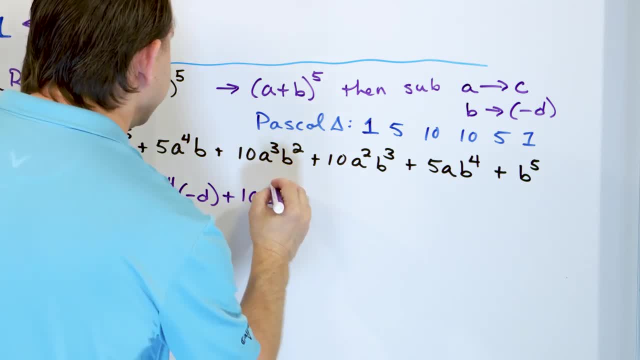 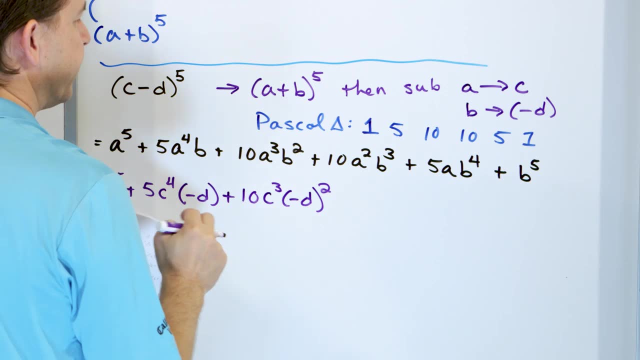 Then I have a 10. a becomes c, c cubed. b becomes negative d. Negative d is squared because b squared. I put a negative d there. Then I have 10. This is going to become c squared. This is going to become c squared. 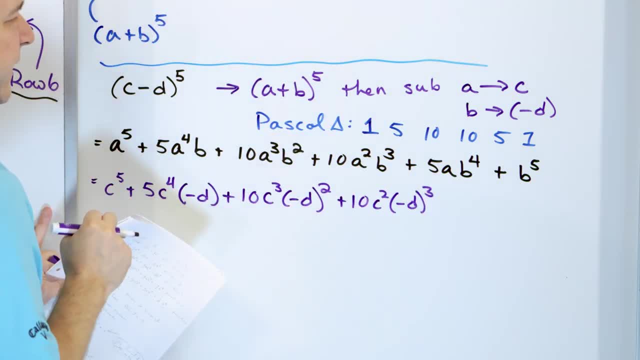 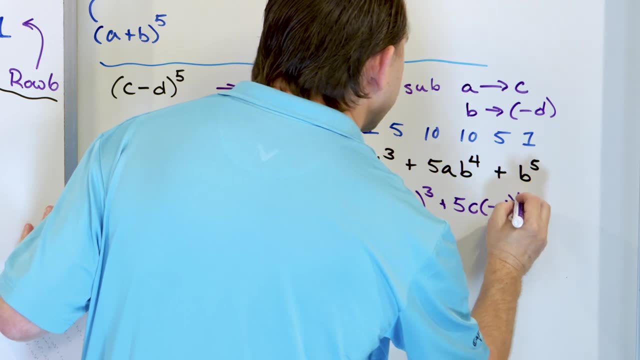 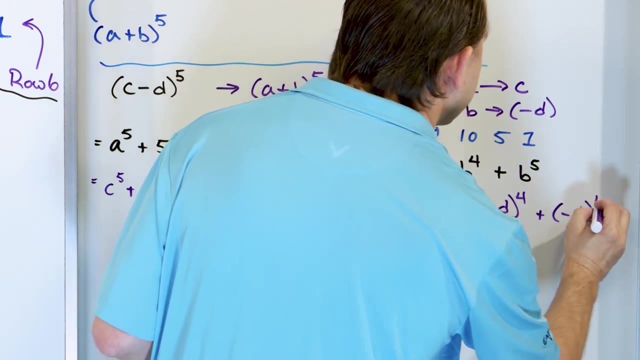 Negative d cubed, because b is now negative d. Then I have 5.. a is c And then I have negative d to the power of 4. Last term here is just b here, So it's just going to be negative d to the power of 5.. 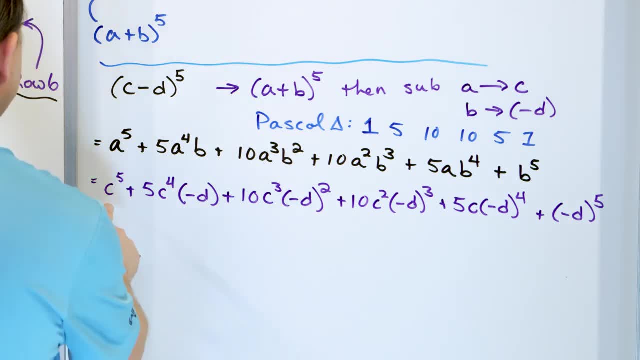 And now I think I'm ready to write the final answer. So here I have: c to the power of 5. This negative sign is going to come out front. Negative 5c to the fourth d. Then notice, here this is going to be squared. 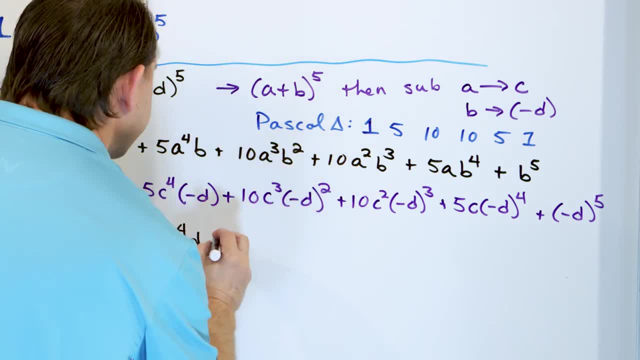 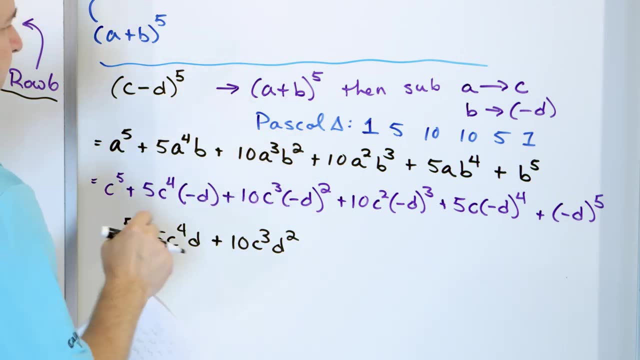 So the negative d is going to be squared, So it'll be positive d squared. So really that sign goes away. So it'll be 10c cubed d squared. The negative sign goes away, But this negative sign doesn't, because it's an odd power. 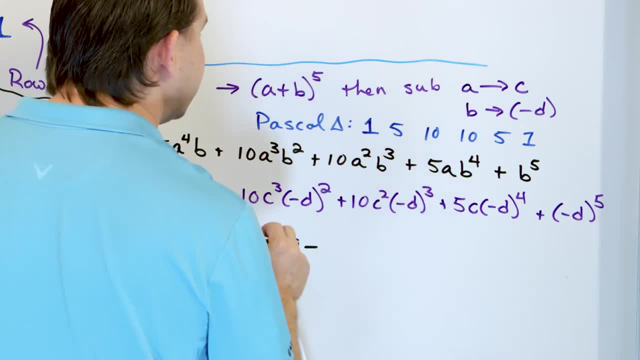 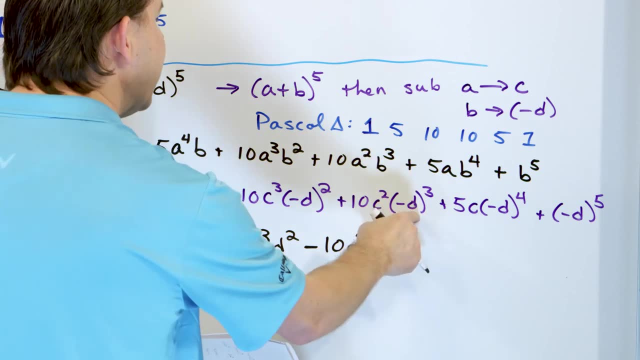 So negative d times, negative d times, negative d. you're still going to have one minus sign that comes out here: 10c squared, But d is still cubed. This negative comes out because of the cubing And d, of course, is still cubed. 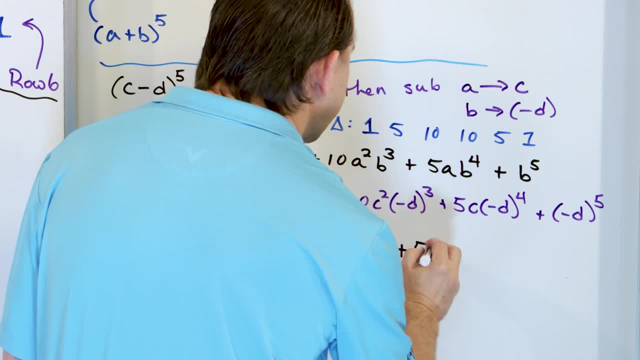 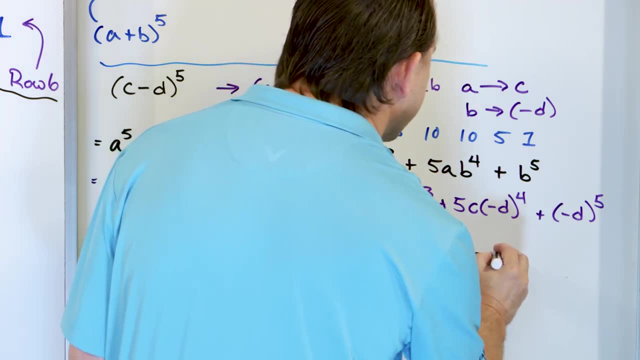 But this is an even power, So this sign goes away. So you have 5cd to the power of 4.. And then this is an odd power, So its negative sign will survive And you'll have d to the power of 5.. 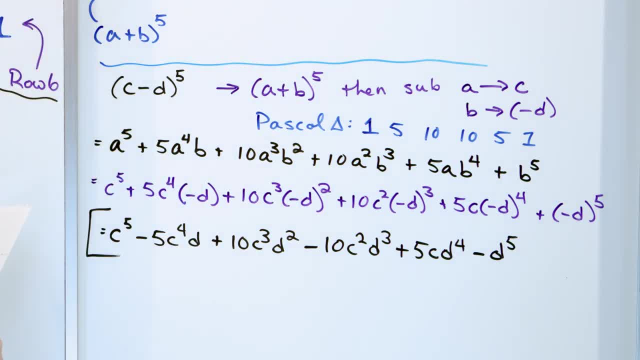 So I'm going to check myself, But this is the final answer: c to the fifth, minus 5c to the fourth: d plus 10c. cubed d. squared minus 10c. squared d, cubed plus 5c. d to the fourth. 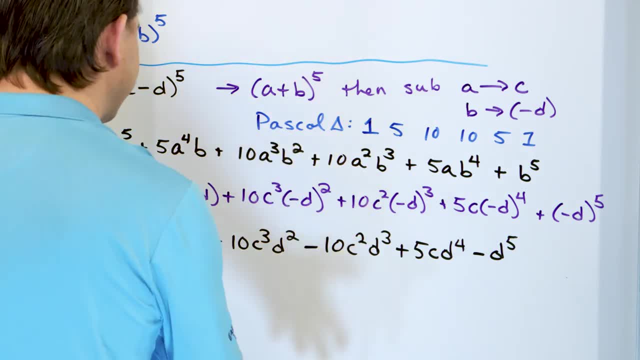 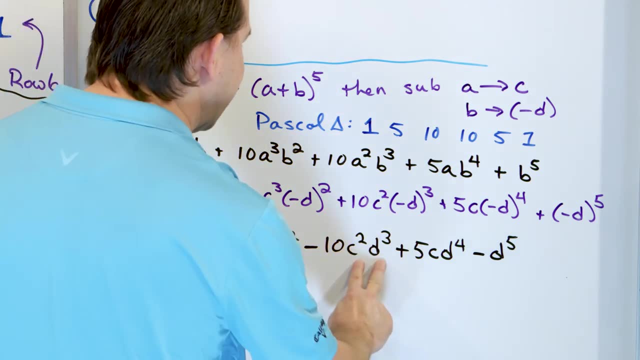 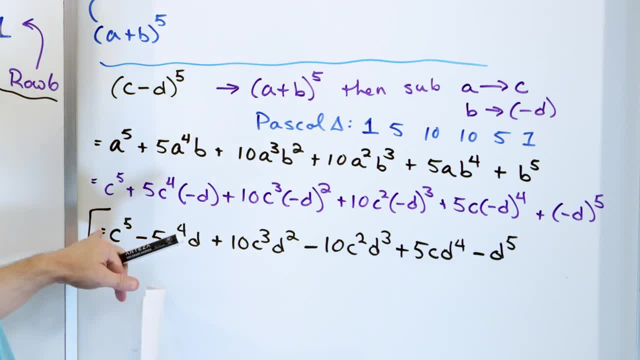 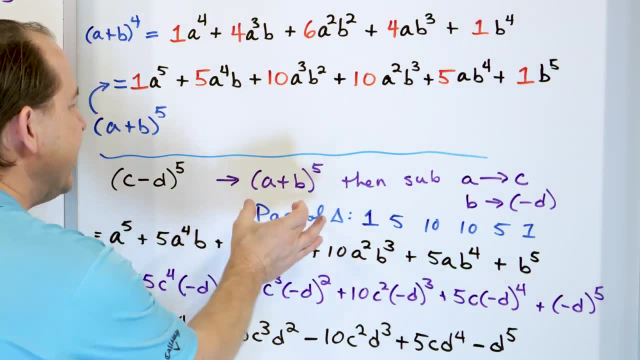 These add to 5. And then that one, of course, adds to 5.. Now the coefficients look a little different than what's in Pascal's triangle. You have negative and positive alternating signs, But that's because we really didn't solve this problem. 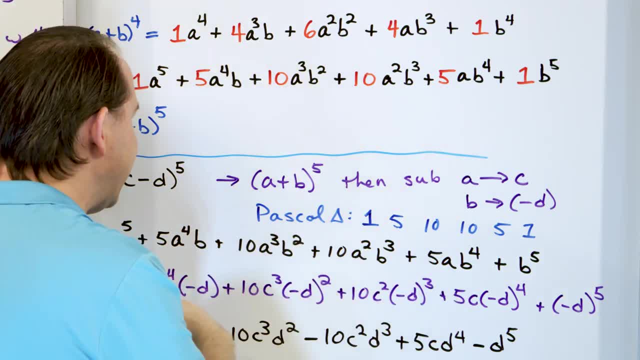 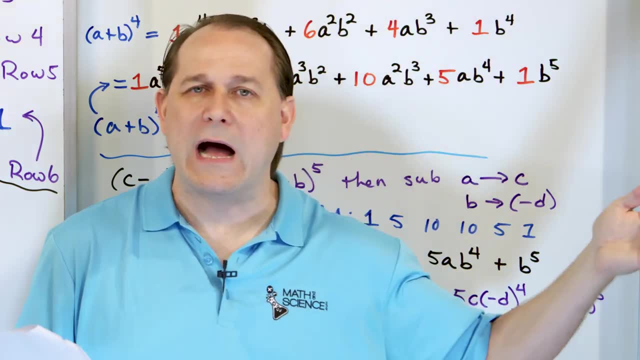 The problem we wanted was this one. So this negative sign is going to ripple through and cause an alternating sign, And that's something you're going to see a lot when you have a minus a minus b or x minus y raised to the power of something. 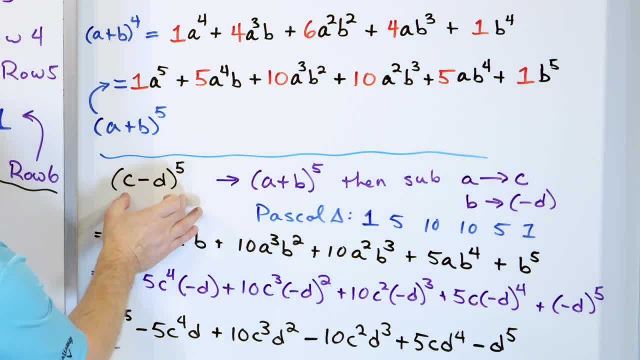 Often you'll see these alternating signs in the final answer. If you did this manually, it would be a nightmare. You'd have to multiply it by itself five times. You'd have so many negative signs to keep track of. But ultimately, if you went through all of that process, 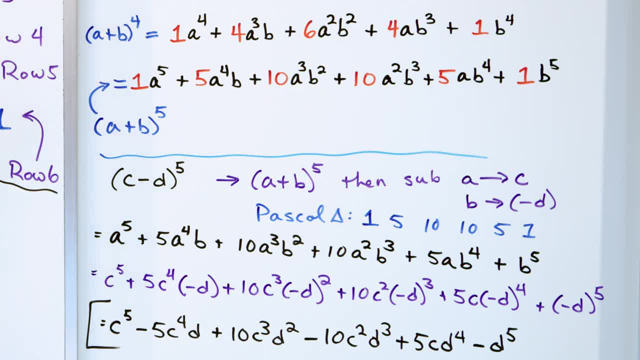 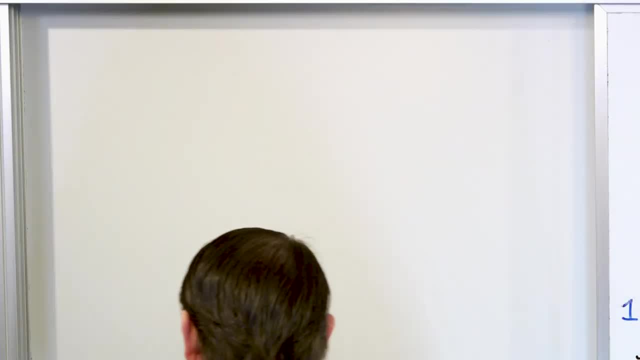 you would arrive at the same answer. OK, Now I have one more problem I want to do. Do I have room? Where do I have room? Yeah, I have room right here. One more problem I want to do: I want to generate the following or expand: 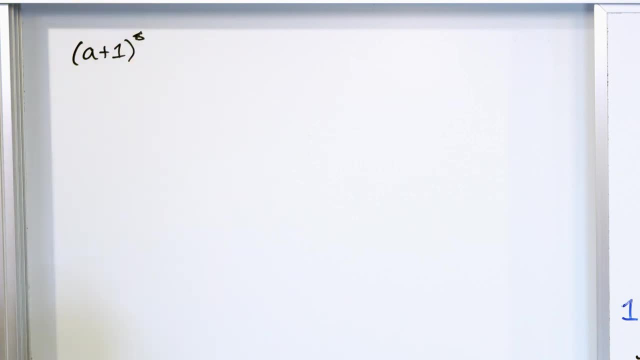 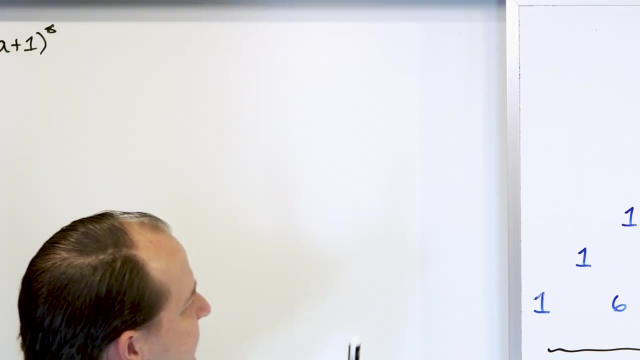 A plus 1 to the eighth power to the eighth power. All right. Now the problem is, since it's to the eighth power, you need to have a row number 8 of Pascal's triangle, right Row number 8 of Pascal's triangle. 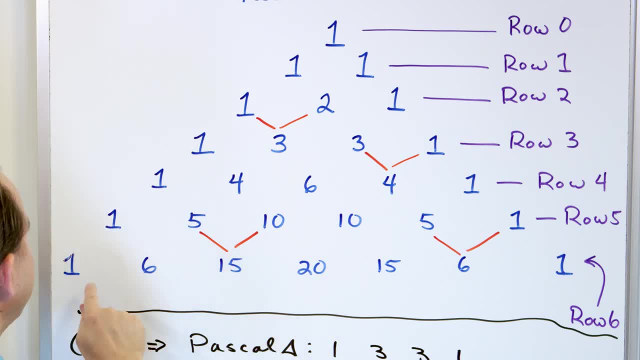 Actually, what I think I'm going to do to make it easy for us is: I'm going to write down row 6 on this page, Because what we need to do is generate two more rows, right? So let's go and do that right now. just to make it 100% clear. 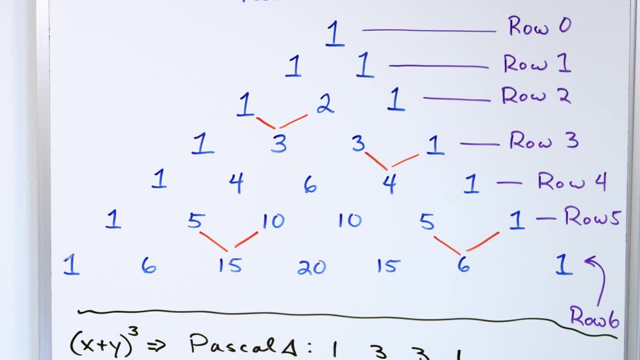 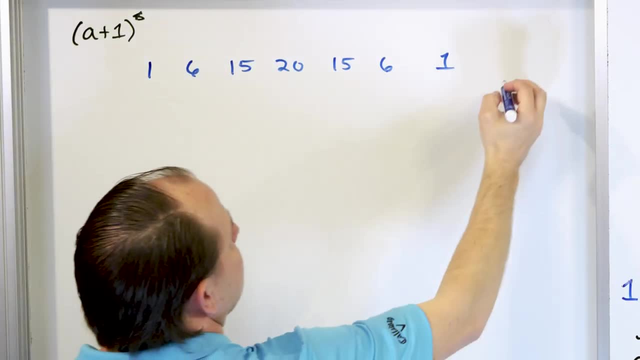 So that row So right there above is 1, then 6, then 15,, then 20,, then 15,, then 6, then 1.. This is row number 6. Row 6.. So we need row 7 and row 8.. 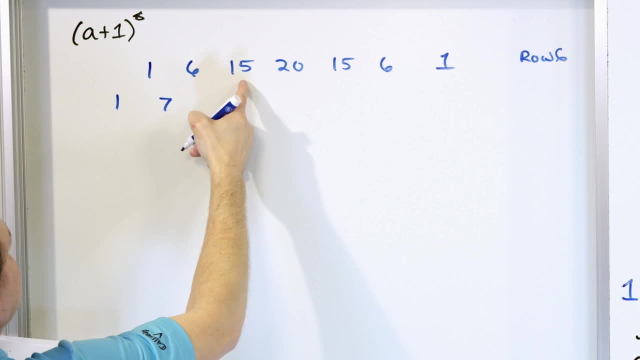 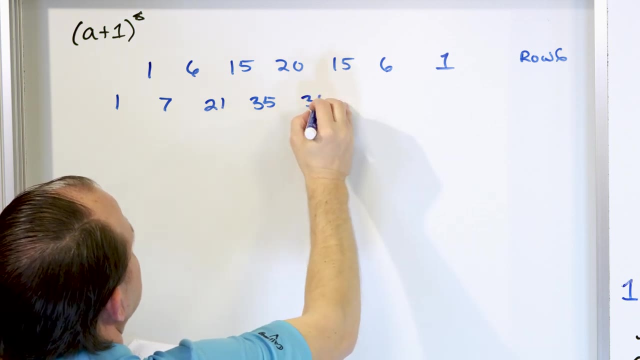 So now we have to put a 1 out here. 6 plus 1 is 7.. This becomes 21.. This becomes 35.. This right here again becomes 35. This right here becomes 21.. This becomes 7.. 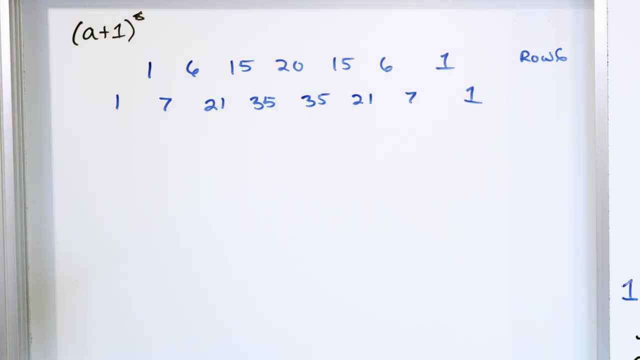 And then the 1 out at the end. So I have 1,, 7,, 21.. 21,, 35,, 35,, 21,, 7, 1.. This is row 7.. This is what you would use if it were to the seventh power, but it's not. 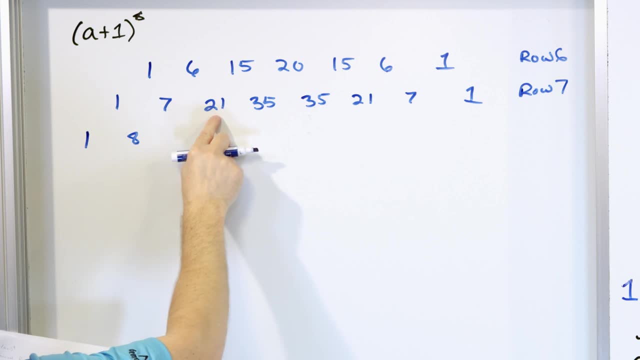 So we have to do one more. Then we have an 8.. 7 plus 21 is 20.. Let's see here: 7 plus 21 is 28, like this: So we have 8 and 28.. Then here we have 56.. 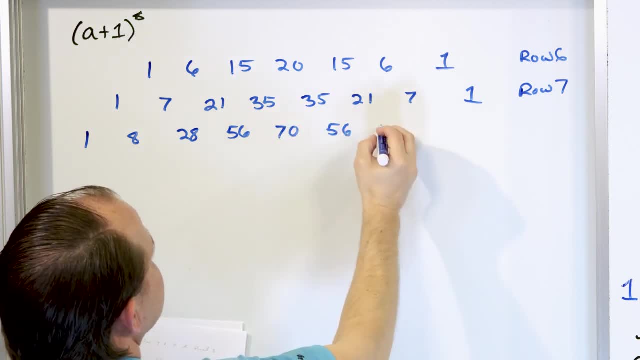 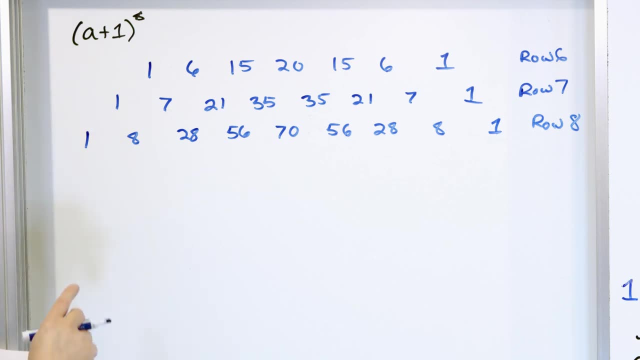 This becomes when we add them 70. Then this becomes 56. Then this becomes 28.. Then this becomes 8. And this becomes 1.. This is row 7. 8.. So let me double check: 1,, 8,, 28,, 56,, 70,, 56,, 28,, 8, and 1.. 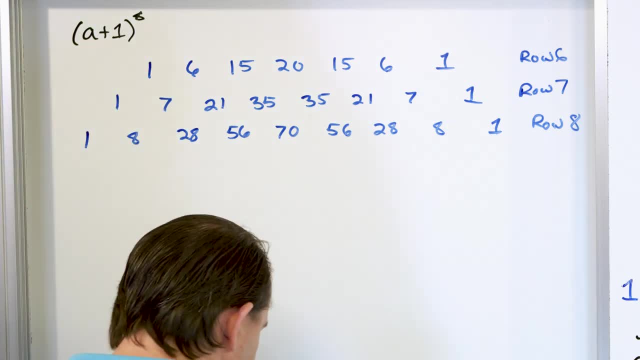 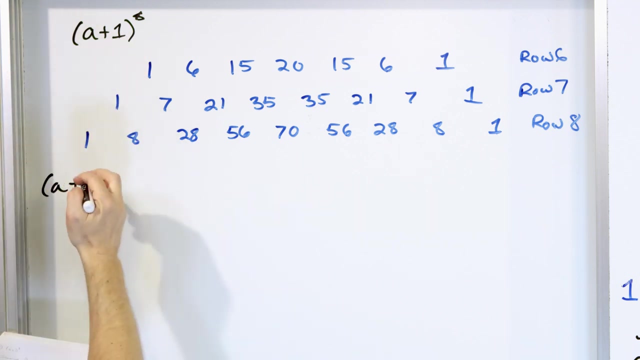 So now we have what we need to generate an expansion which is a monster to the eighth power like that. So what do we do next? So we say that a plus 1 to the eighth. So what we want to do is just go ahead and do a plus b to the eighth. 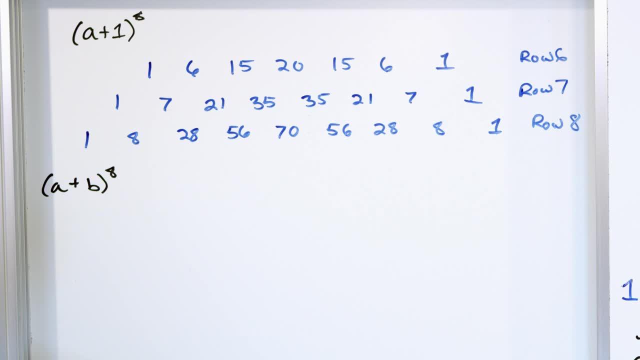 And then, at the end of it, we'll just substitute and make b equal 8.. And then, at the end of it, we'll just substitute and make b equal 1. That's the easiest way to do it. So what do we do? 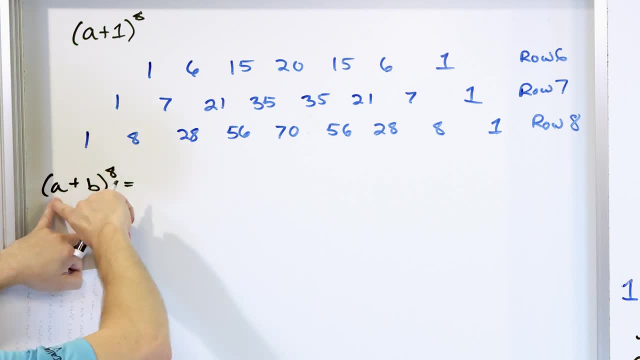 We first say we need this row, We need a 1.. And then the first term is going to be a to the eighth power. So a to the eighth power, like this, Next term is going to be 8.. Then what do we do? 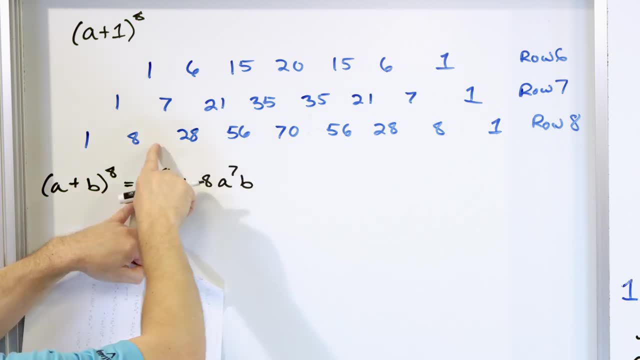 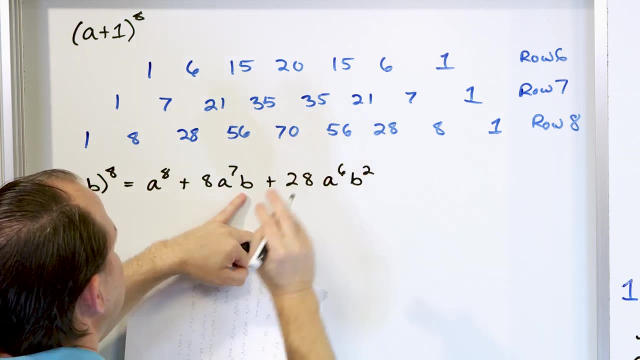 a comes down to 7, and b goes up to 1.. Then it's going to be 28.. Then what happens? a comes down to a 6, and b goes up to a square. After 28 comes 56.. 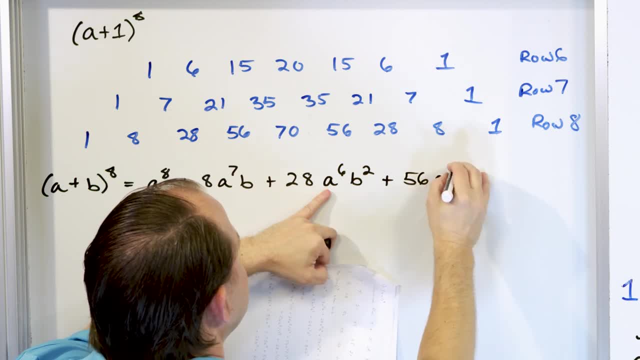 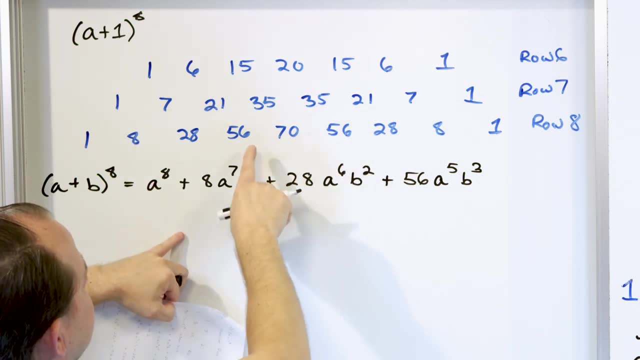 56. Then what happens? a comes down to the fifth and b goes up to the third. Now I've got to go to the next line here. So after 56, let's see here, That was this 56.. I have a 70. 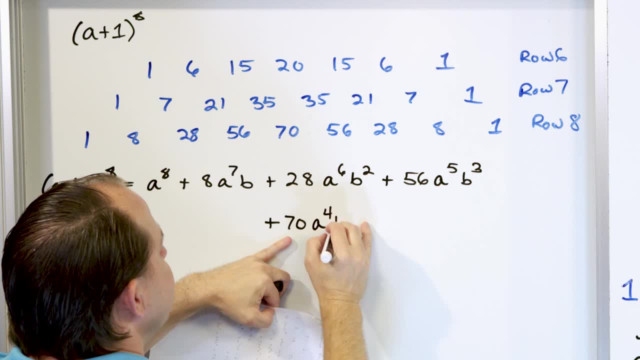 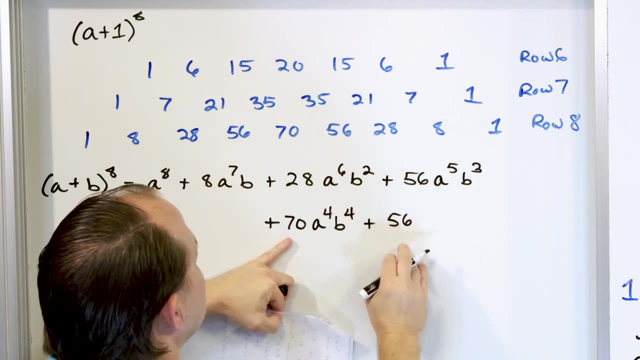 And then a 70 is going to be a coming down to the fourth b. going up to the fourth, That's 70. Then I have a 56. And the 56 is going to be a cubed b to the fifth. 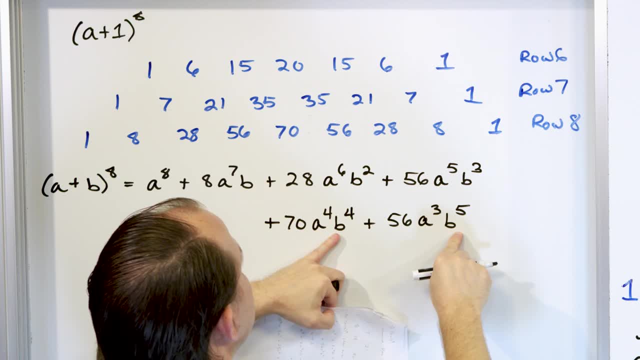 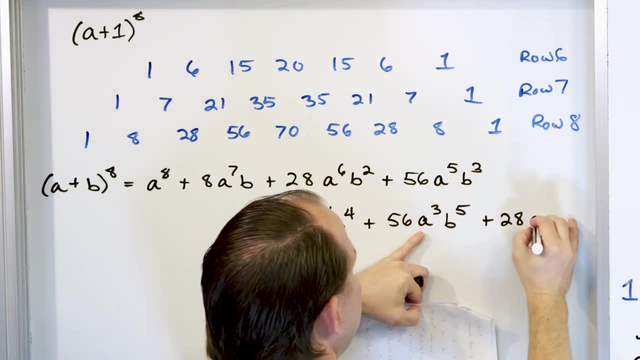 Again coming down in a and up in b, And then I'm going to have after 56, 28.. I should have given myself more room here. it looks like I'll have an a squared b to the sixth, down in a and up in b. 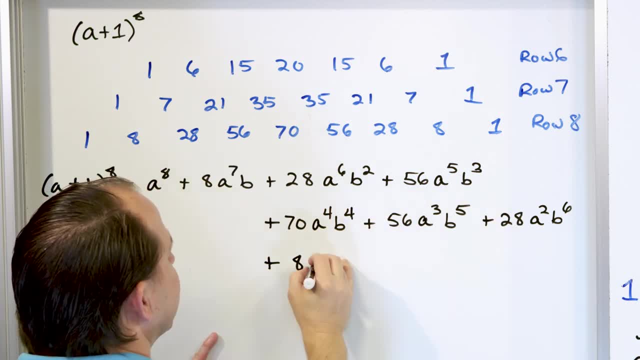 And then after 28, I'm going to have an 8. I'm going to go down in a and up in b, And then I have a 1. And then down in a is a to the 0, so it goes away. 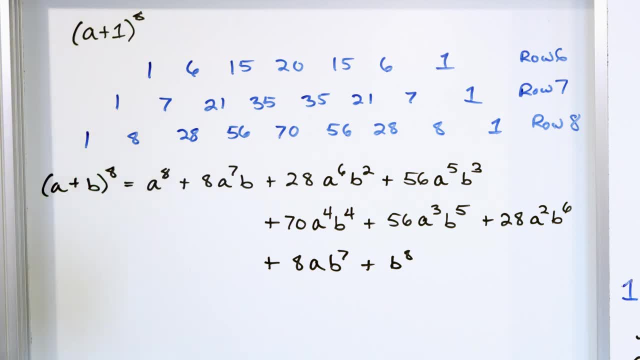 And then b to the eighth power. So let me double check myself: 88, a, 7, 8 a, 7 b And then 28 a to the 6.. to the sixth, b squared, then plus 56, a. to the fifth, b, cubed, then plus 70, 4 and 4,, 56, 3 and 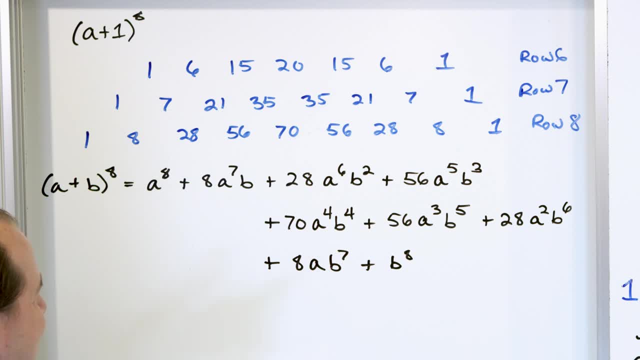 5,, 28,, 2 and 6, and then 8,, 1 and 7, and then b 8.. And you should just kind of scan and make sure these exponents should always add together to be 8 for every one of these terms, Everywhere you. 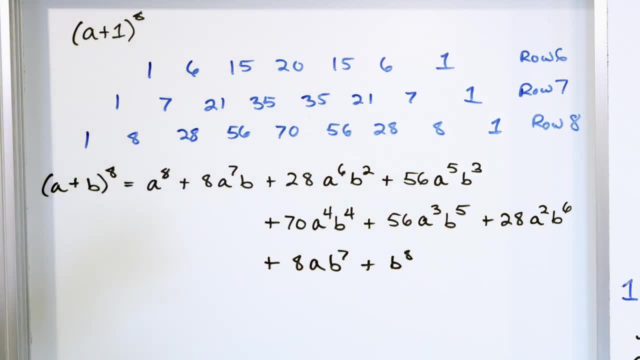 look, it should always add to 8,, and that's always true of any kind of polynomial expansion like this. Okay, so if we were asked to find this, it would be simple, but we're not. We want to find this, so we want to set b equal to 1.. So what do we do there? It's just exactly like it sounds. 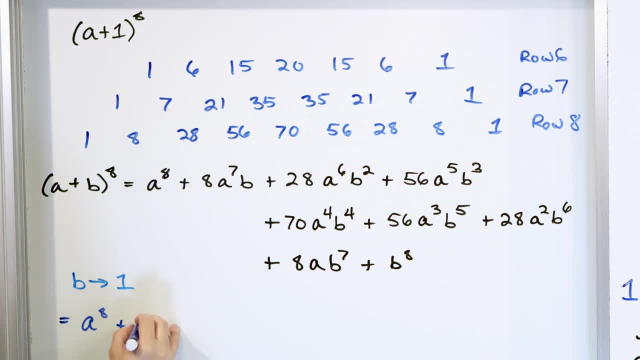 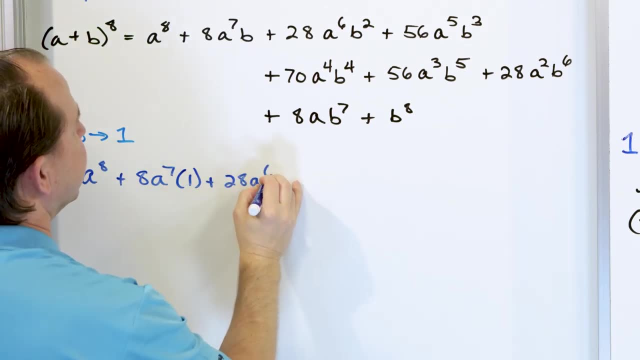 a to the eighth is right here, then we have 8, a to the seventh, but then we have b. so just put a 1 right there, Then you'll have 28, a to the sixth, then you'll have 1 squared. putting a 1 in for. 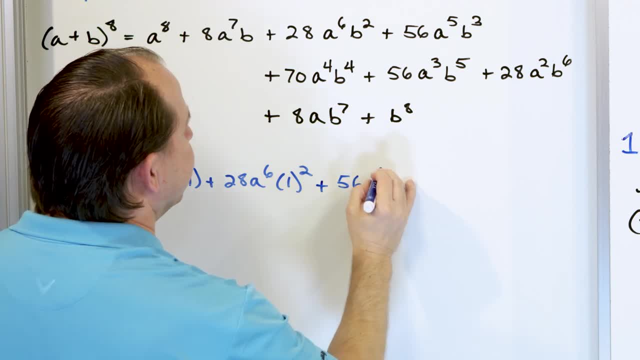 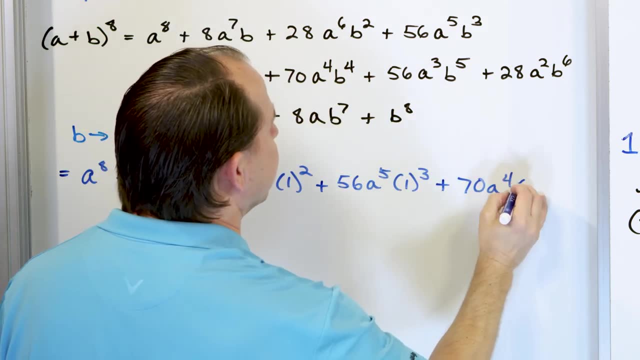 this b, Then you'll have a 56, a to the 5th- 1 cubed putting a 1 in for this. Then you'll have a 70, a to the 4th, then 1 to the 4th, putting a 1 in here. Let's go way back over here. After 70 becomes. 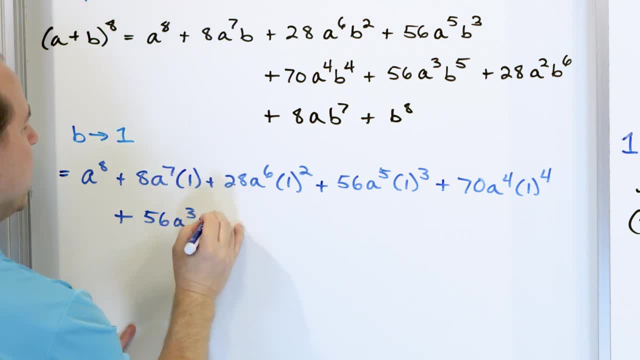 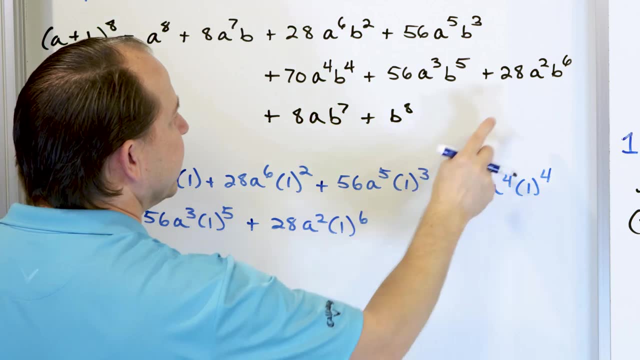 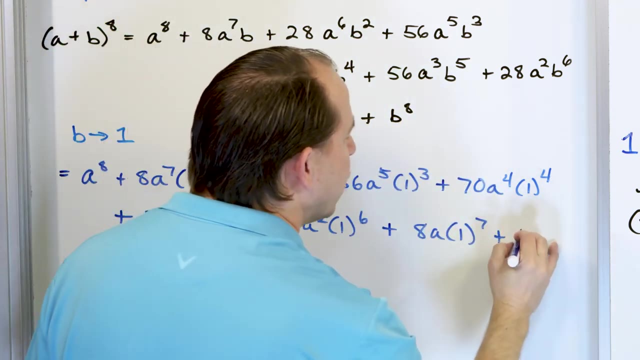 this one, 56, a cubed 1 to the 5th- this one. Then we have a 28,. a squared 1 to the 6th right here. Then we have an 8, a 1 to the 7th. Then we have b becomes 1, so it's. 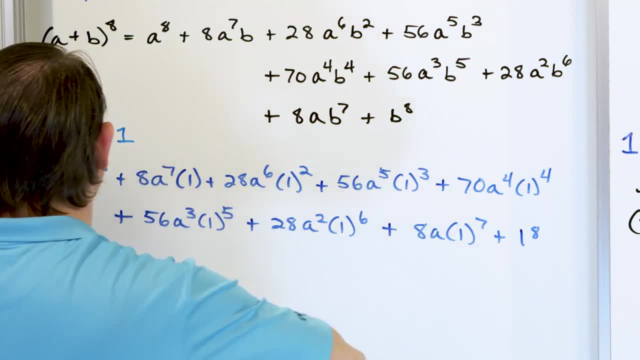 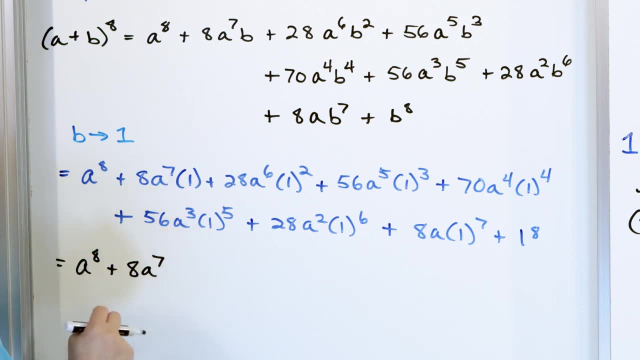 1 to the 8th power. So finally we're almost done. I know it's a ton of work, but we're almost done. We have a to the 8th power. This is just a 1, so we have 8, a to the 7th. Then 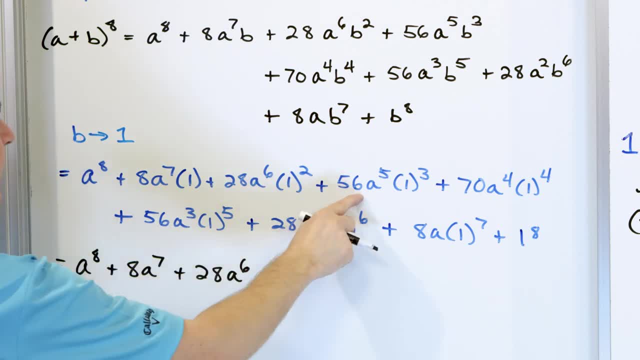 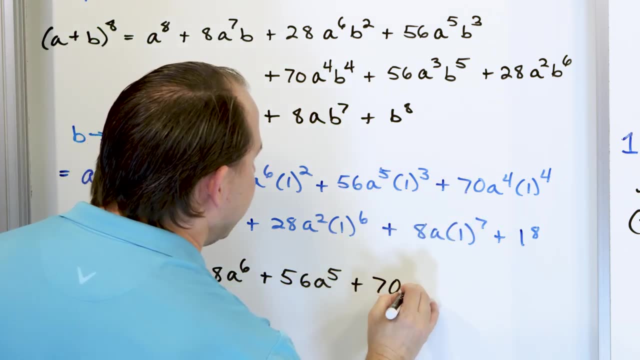 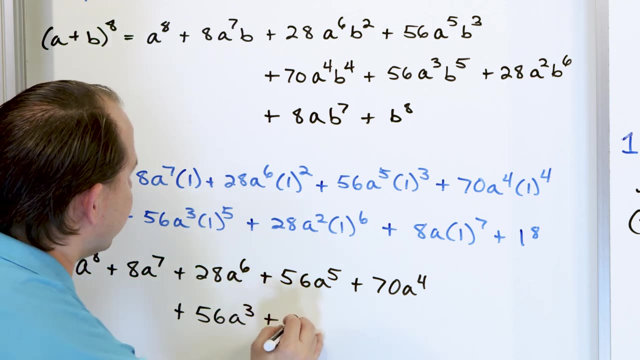 we have 28, a to the 6th, Then we have 56, a to the 5th, Then we have 70, a to the 4th, Then we have 56.. I'll start over here: 56, a cubed, then 28, a squared, then 8, a, then 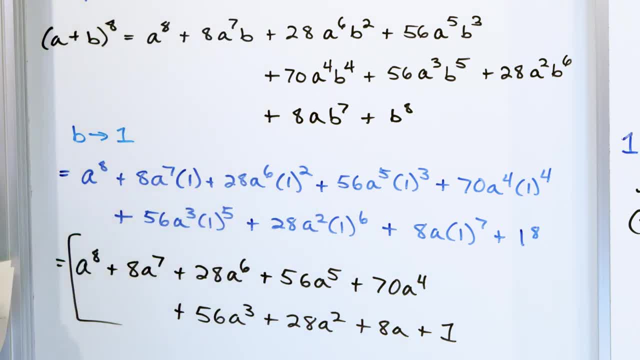 1. Just writing all of these down here. This is the final answer. Let me double check: 8,, I'm sorry. a to the 8th power 8,. a to the 7th, 28,. a to the 6th, 56,. a to the 5th. 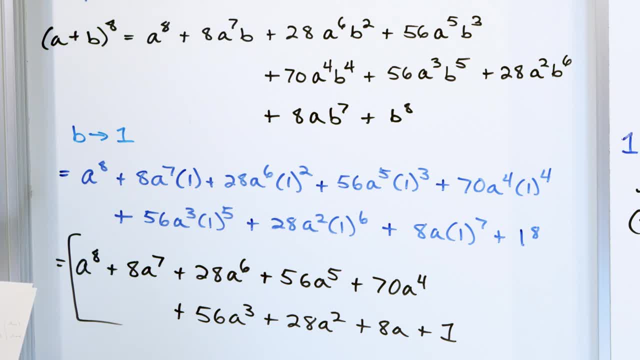 70, a to the 4th, 56,, a cubed 28,, a squared 8a and 1.. This is the final answer. So you can see that it is a 1 to the 6th power. 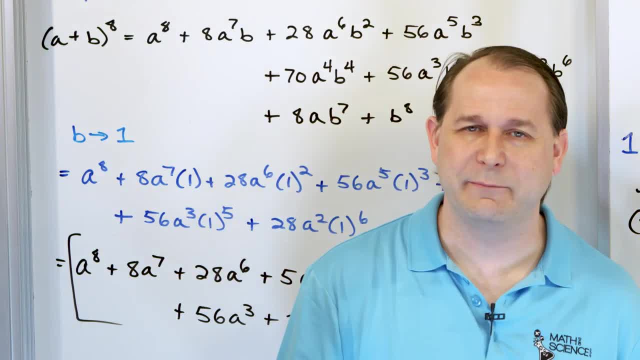 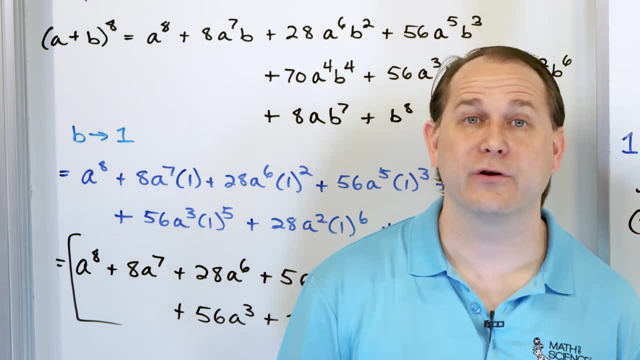 This is still work to apply Pascal's Triangle to expand binomials. but it's way less work than actually multiplying all these terms out and actually adding them all together, canceling terms if needed and collecting everything, all the while trying to make sure. 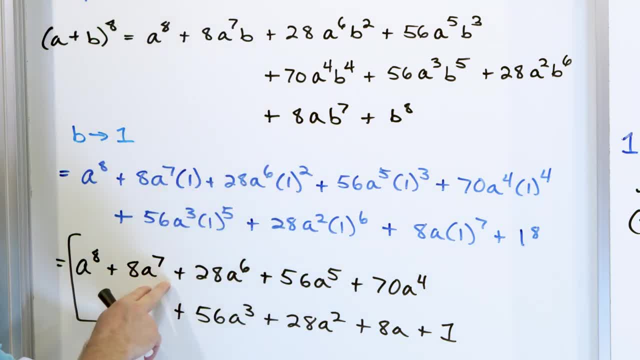 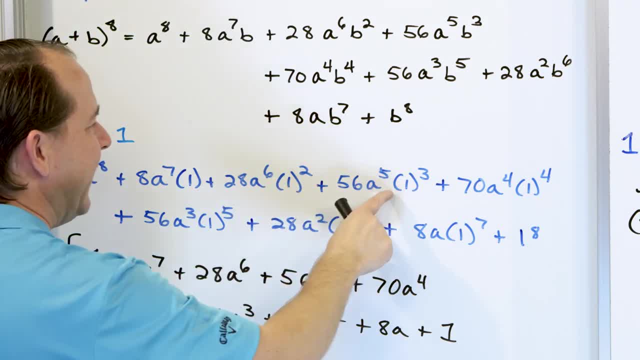 1 to the 1st power. You have an invisible 1 to the 1st power. These exponents do add up to 8.. These add up to 8.. These add up to 8.. It's just that it doesn't show up in the. 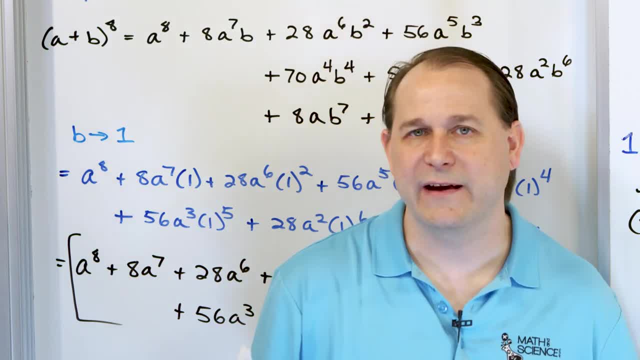 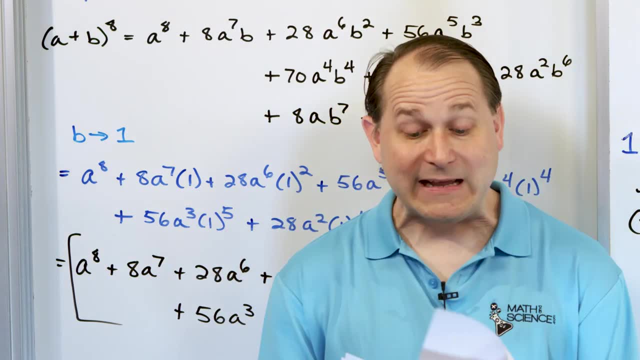 final answer, because we've evaluated and kind of calculated some of those exponents, So of course they don't show up all the time in the final answer. This is how a computer might do it, or one way in which a computer might do it. So what I'd like you to do is: 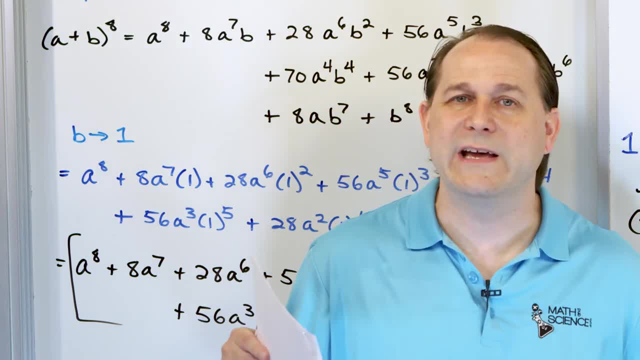 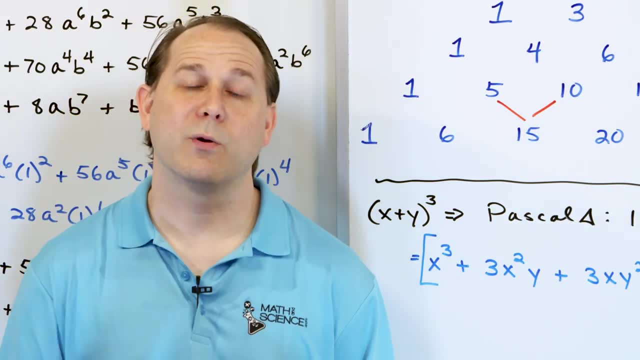 sit down with a piece of paper and convince yourself by doing these problems that you can get the answers that I get. Do it yourself. There's no substitution for you doing it yourself. Then follow me on to the next lesson. We'll get a little bit more practice with evaluating. and expanding binomials using Pascal's Triangle.